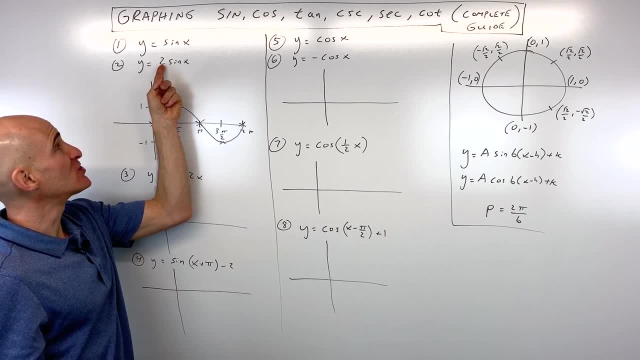 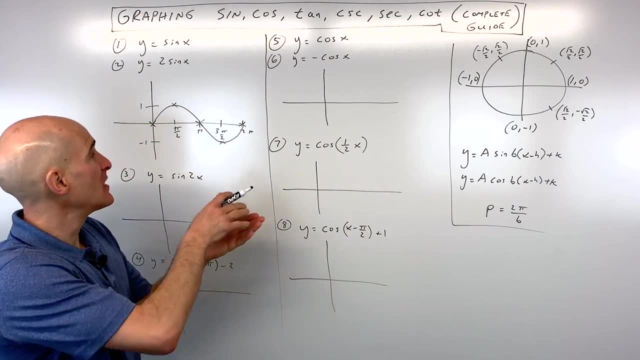 at negative one. Now, what happens if you wanted to graph: y equals two times sine of x. Well, this number that comes in front, this is what we call our amplitude, and this is what we call our amplitude A, and that's going to be a vertical stretch of two. So what happens is, instead of going up to one, 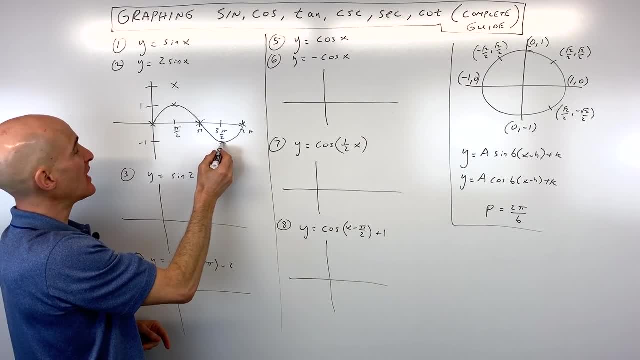 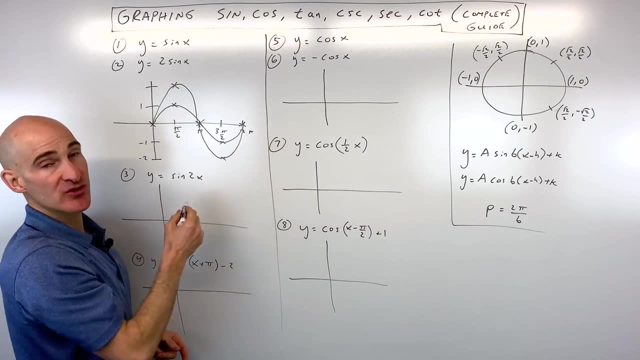 now you're going to go up to two, Instead of going down to negative one, you're going to go down to negative two, and so, again, that's just a vertical stretch, but it's still going to cross the x-axis at those same points. So now let's see if we want to go to a slightly more challenging problem. Say: 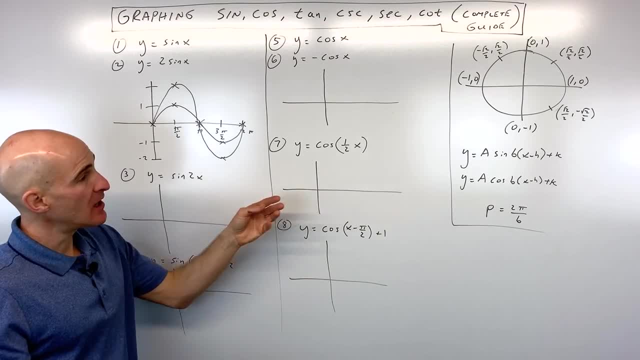 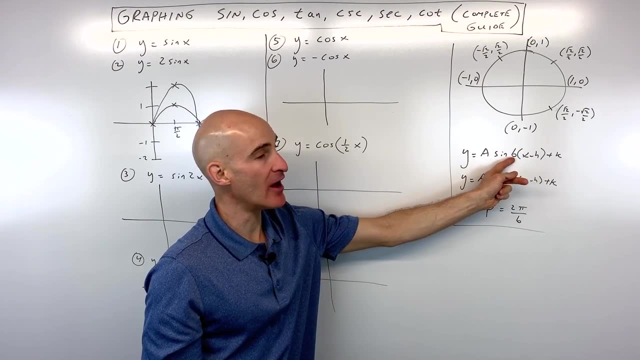 like number three. we have: y equals sine of 2x. This number here, okay, this b value, the letter that comes or the variable or the constant. I should say that comes before the variable x. that b value affects the period and we can use this formula: period equals 2 pi over b to find out. 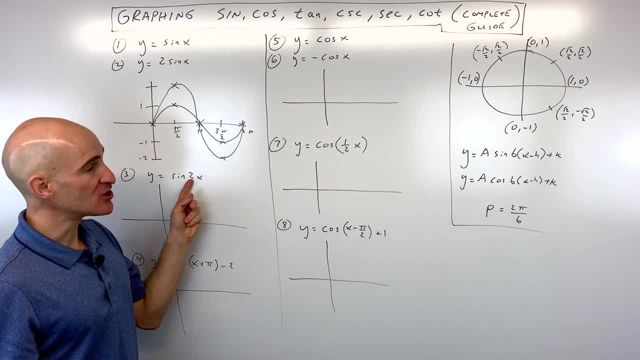 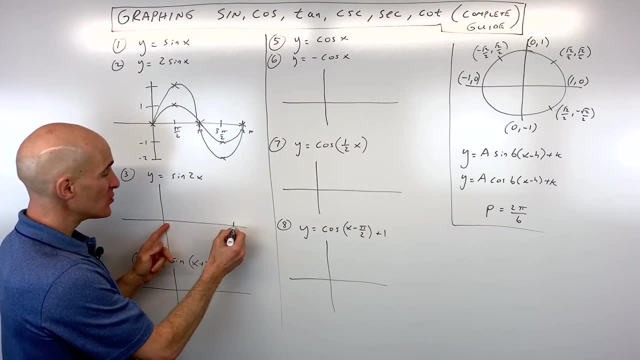 what that new period is. So in this case the b value is 2.. If we take 2 pi divided by 2, that's just going to be pi, So our period is going to be pi. What I like to do is I kind of like to mark 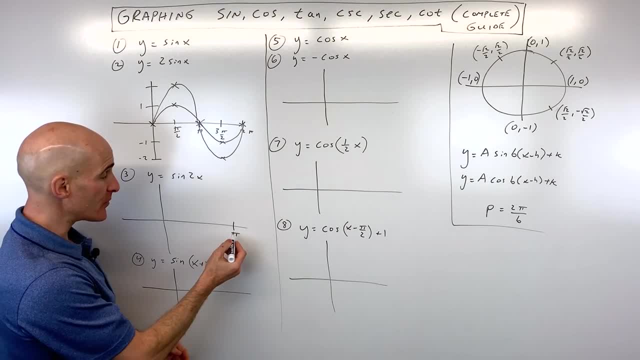 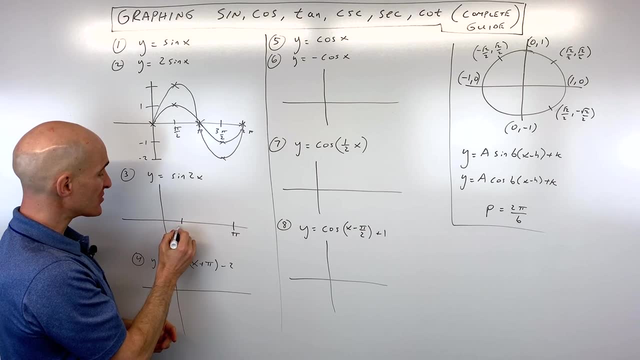 the x-axis, the scale first. If the period is pi, I'm going to divide it up into four pieces, just so we did here. one, two, three, four. So pi divided by four gives us our scale. that's going to be pi, pi over four, two, pi over four, three, pi over four, four, pi over four. okay, so two pi over four, and 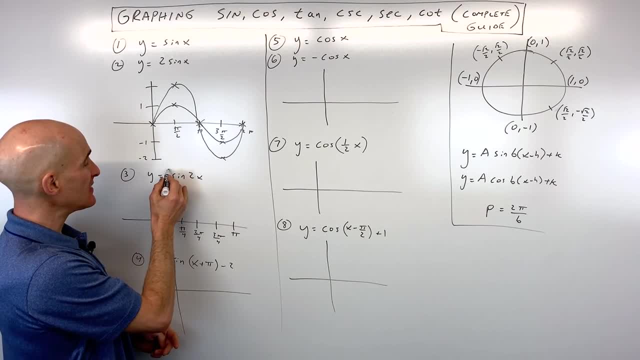 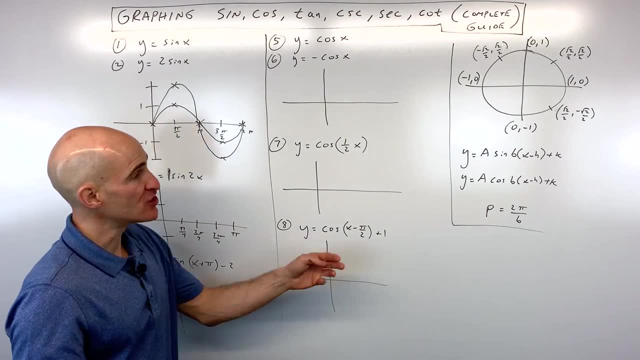 three pi over four and four pi over four is pi. We can see that the amplitude is one, because one times anything is itself. so it hasn't been stretched vertically at all and we haven't talked about the shifts yet. that's the h and the k that's going to pick up the graph, move it left. 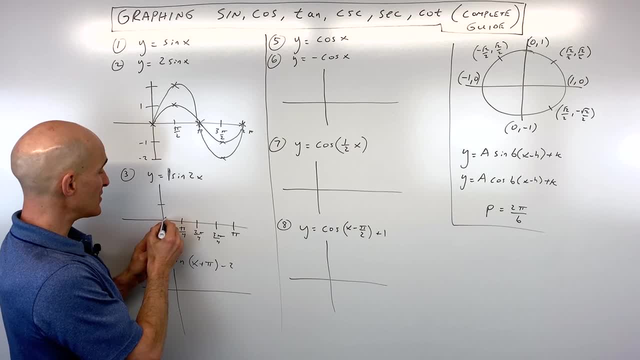 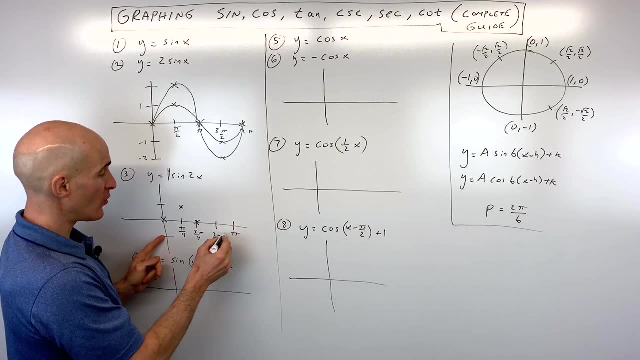 and right up and down. So here we can see that the graph is just going to have this basic shape again. it starts at the midline, it goes up to the maximum, which is one, back to the midline, back down to the minimum, which is negative one, back to the midline. The only thing that was different here is that the 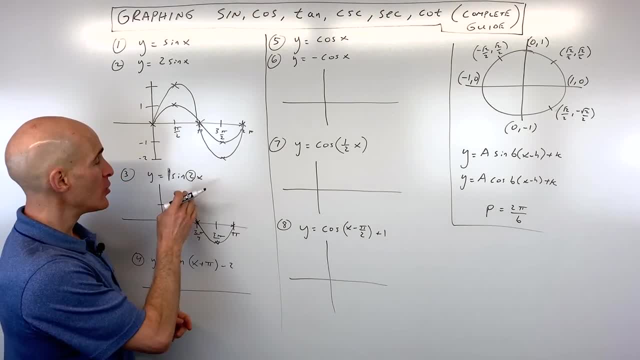 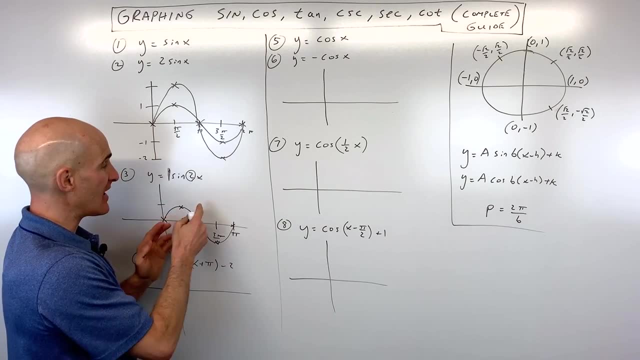 period changed. it was two pi divided by two, which is pi. Notice, though, that this number- here it has the opposite effect on the graph. instead of multiplying the x's by two, we actually divided the x's by two. Normally, the period for sine and cosine is two pi. here it would divide the x's by. 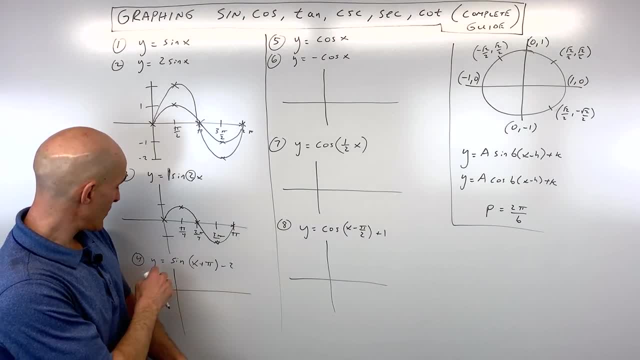 two. the period was just one pi. So let's keep going. so let's go to number four here. now we're getting into: y equals sine of x plus pi minus two. So here you can see that we're going to see that the b value is one, so which means that our period is two pi divided by one, which is just. 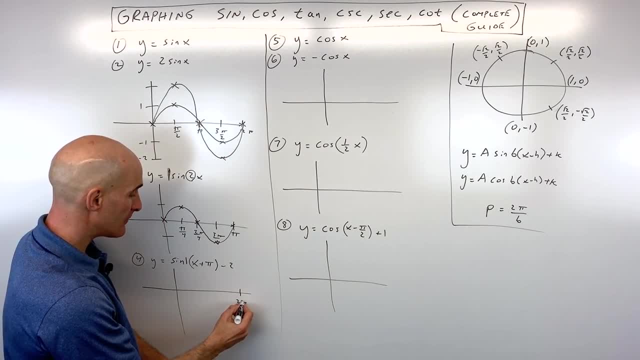 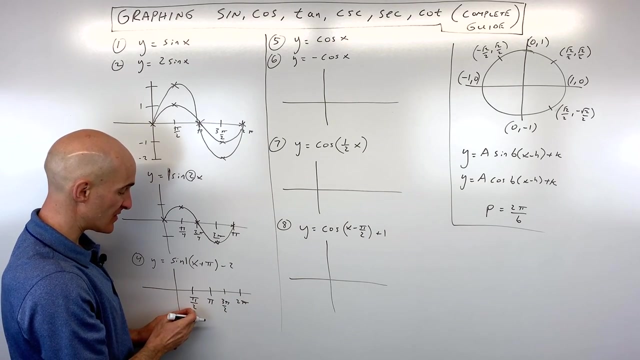 two pi. so let's go ahead and mark our scale here. two pi divide it up into four pieces: one, two, three, four. if you take two pi divided by four, that comes out to two pi over four, which reduces to pi over two, two pi over two, which is pi, three pi over two, four pi over two. so i'm just taking this pi over. 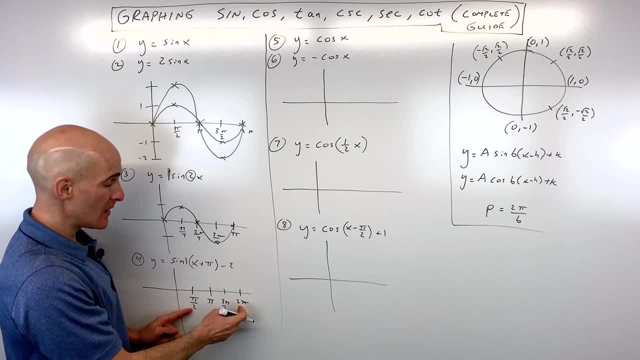 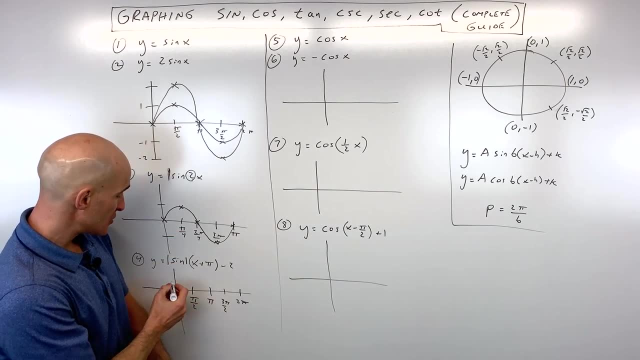 two, multiplying it by two or by three or by four, and that's how i'm getting the scale. on the x-axis, The answer is that the b value is one, so we're going to take the b value and we're going to go down to the x-axis, So the b value is one, so it's not being stretched vertically at all, so that 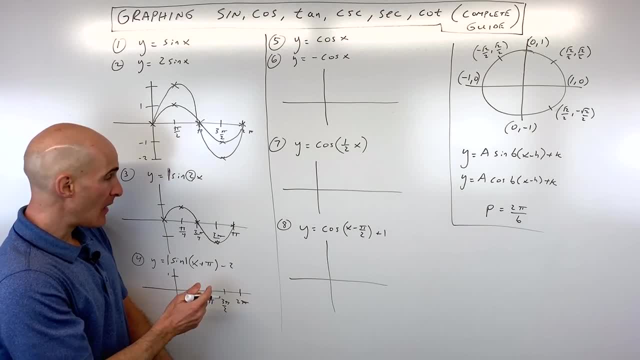 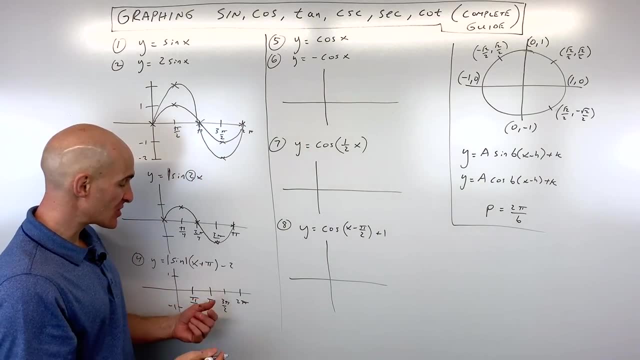 means it's going to go up to a maximum of one and down to a minimum negative one. but the number, this group with the x that's going to shift the graph in the x direction. it has the opposite effect. so plus pi is actually going to shift the graph: left pi, okay, negative pi and then the minus. 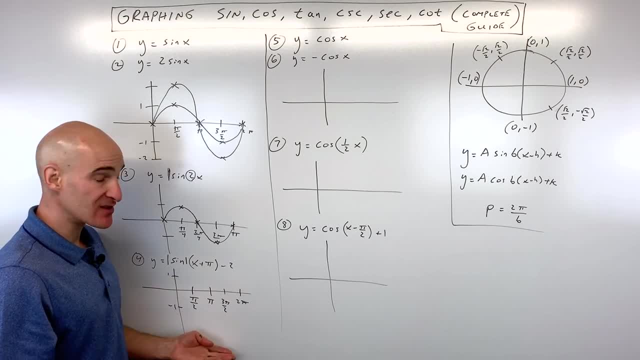 two has the same effect. that's going to be a vertical shift. the minus two is actually going to shift it. the same down two okay as the sine. so what's going to happen here is we can think of: this graph is shifting left pi. now notice how our scale is pi over two. so to shift left pi, that's actually like shifting. 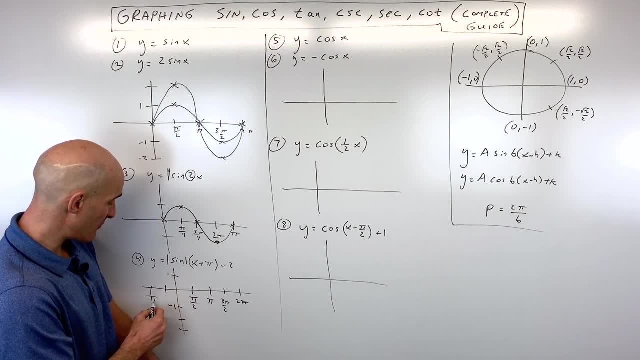 left two steps: one, two. so here we're over, here at negative pi and we're shifting down two. so that's going to be one, two, so that we can think of this point right here as like our new origin, like our new starting point. okay, so i kind of drew like a new y-axis and a new x-axis, and so what i'm going. 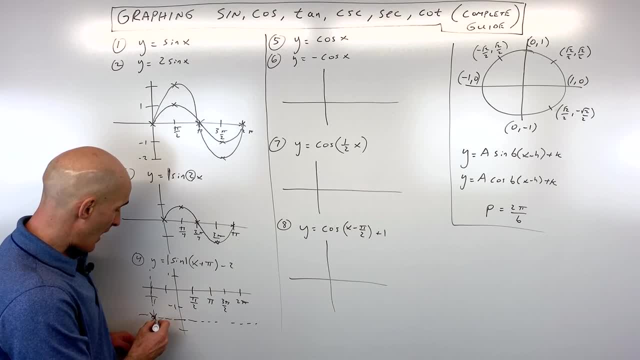 to do now is i'm just going to graph from here. so i'm starting at the midline, i go up to the maximum, which we said was going to be you know one okay, because it's not being stretched at all- back to the midline, back to the minimum and then back to the midline. so that's our basic graph, the only. 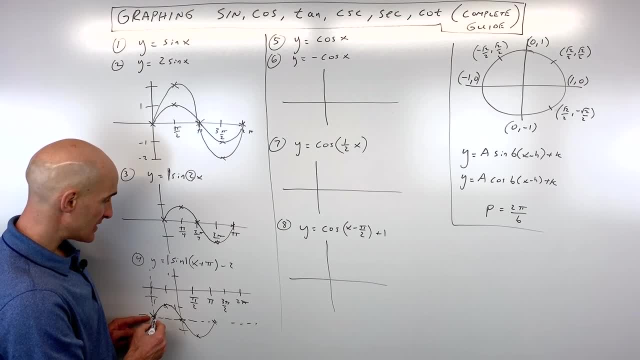 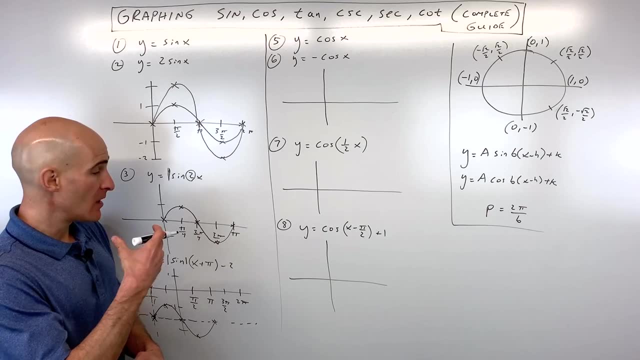 thing we did is we shifted everything left to and down to, and we thought of that as our new starting point. okay, let's talk about cosine. we're going to get into some more challenging examples involving the amplitude changing, the period changing, as well as a phase shift left and right and a vertical 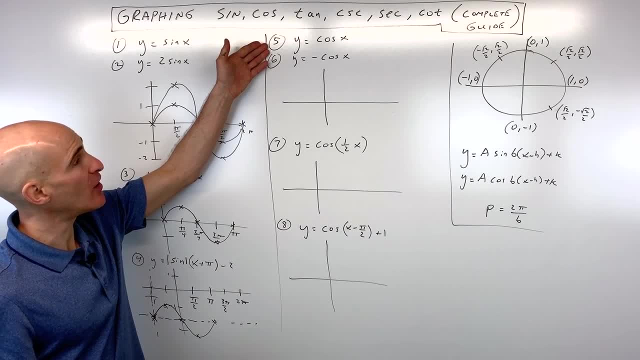 shift up and down. but let's talk a little bit about cosine first. so when we talk about cosine, we're going to get into some more challenging examples involving the amplitude changing the period. cosine: we go to our unit circle, The cosine: we're talking about the x-coordinates. when we 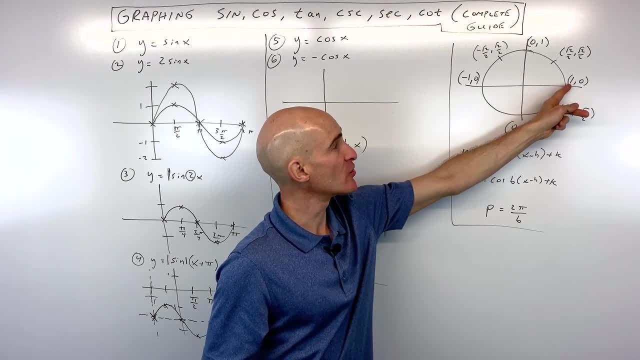 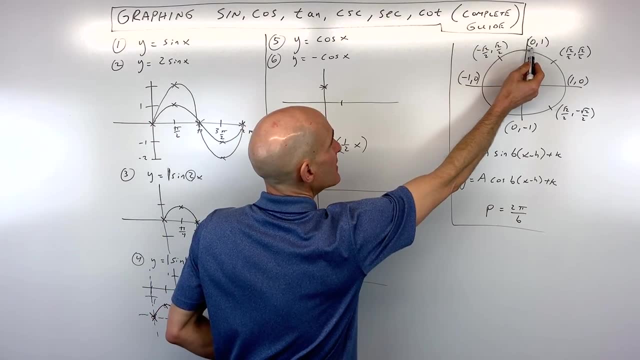 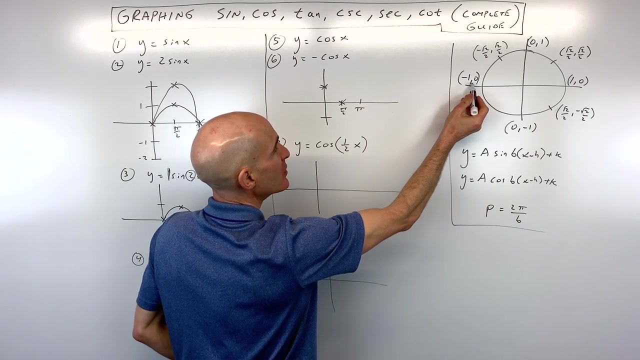 find the cosine values. So cosine of zero degrees or zero radians is going to be one. So with cosine at zero, we start at one. At pi, over two or 90 degrees, the x-coordinate is zero. So we go back down to zero. At pi, which is here at 180 degrees, the cosine is x-coordinates, negative one, And then 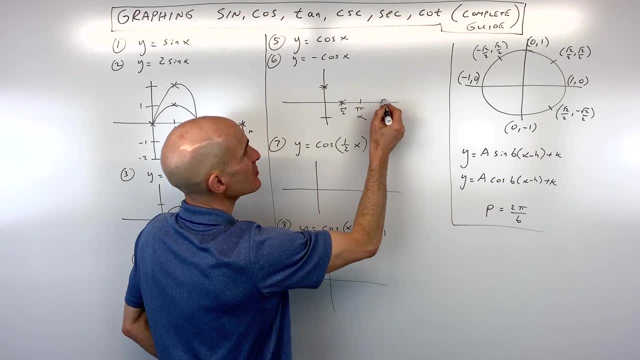 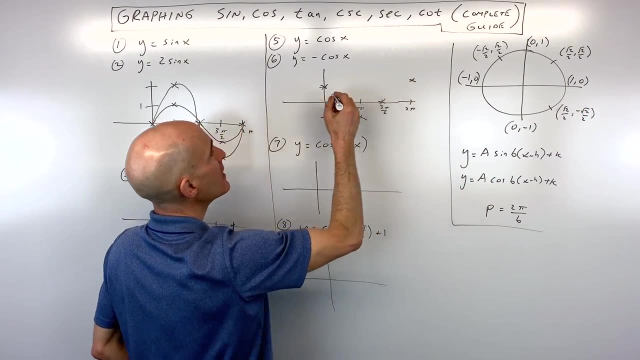 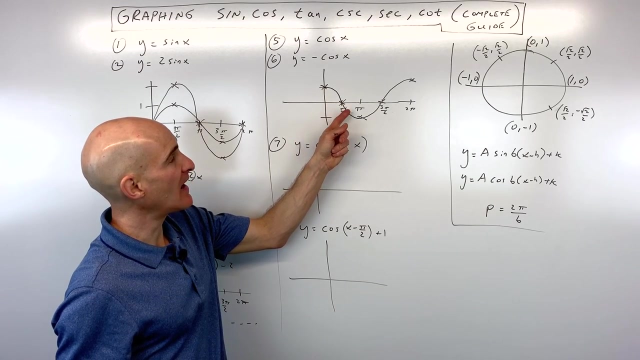 at three pi over two, the x-coordinate is zero. And then at two pi, you're back to where you started. The cosine is x-coordinate, you're back to one. So you can see, our basic cosine graph has that basic shape like that. It starts at the maximum, it goes to the midline, down to the minimum, back to the midline and then back up to the maximum, and then it repeats. So these are called sinusoidal graphs. They have like that s shape. So now, what would the graph look like if you had y equals negative? 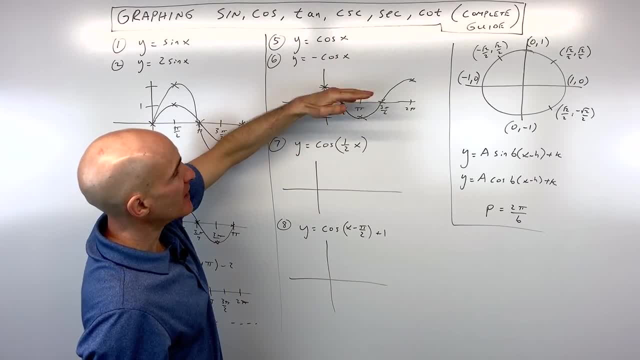 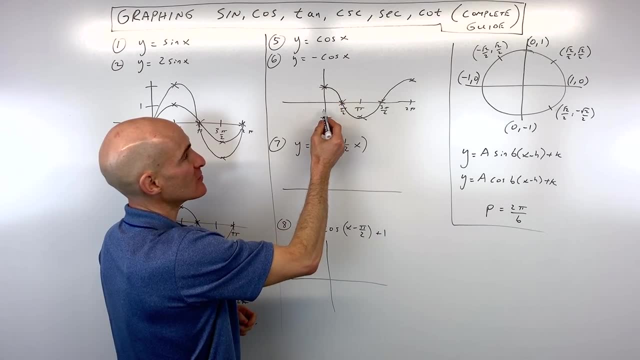 Well, the negative what it does is it reflects the graph over the x-axis, So all the x values are going to be- I'm sorry, all the y values are going to be the opposites The x values are going to be. 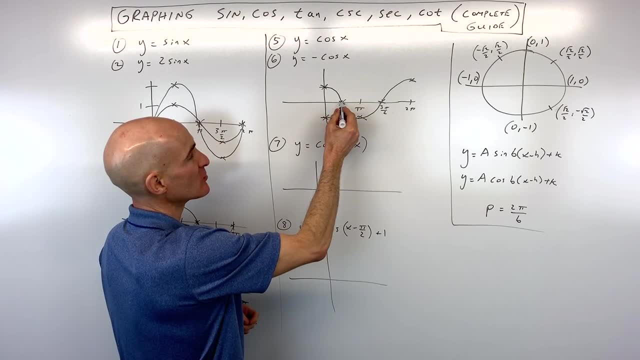 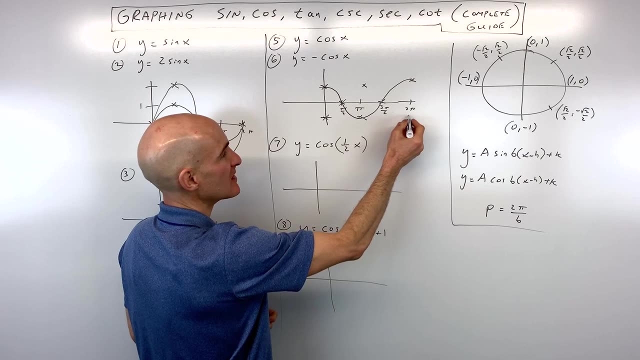 the same. So instead of being at one, you're going to be at negative one. Zero times negative. one is still zero. Negative, one times negative. one is positive one. Zero times negative one is zero, And one times negative one is negative one. Again, we're just reflecting it, So this graph is going. 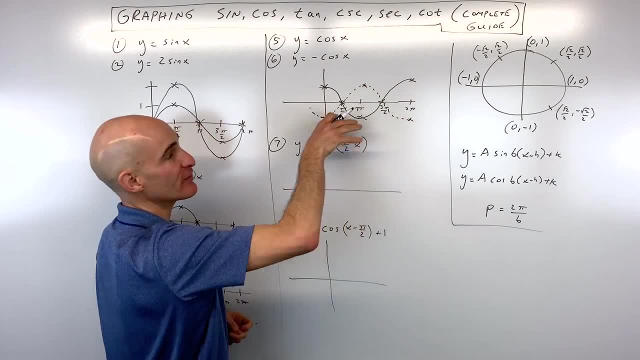 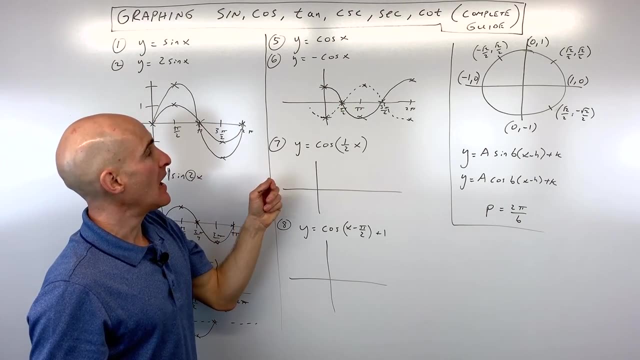 to look something like this dotted line here It's just been flipped Again. you want to remember the basic shape. So cosine has that basic shape. Sine has this basic shape. And let's go to number seven now. Y equals cosine of one-half x. So just like sine, we look at that b value, that number. 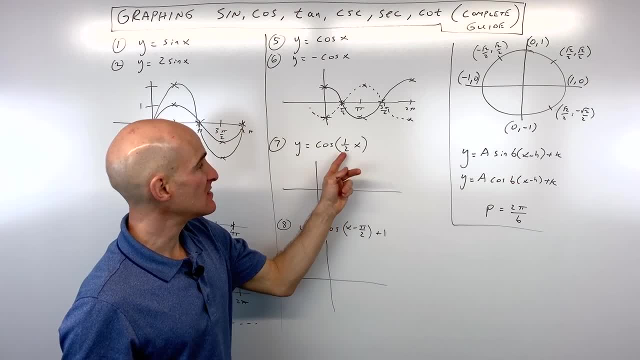 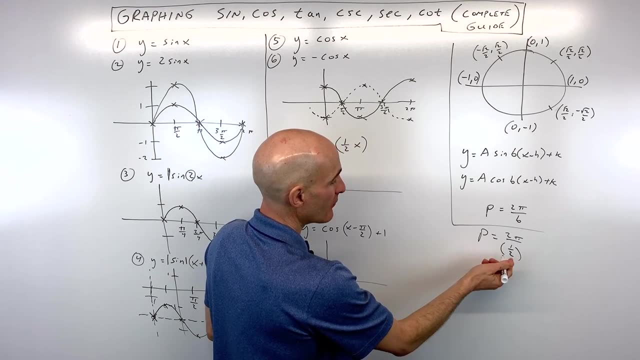 that comes just in front of or to the left of the variable x And we can see that that b value is one-half. If we want to find the period, we just say 2b divided by b, which is one-half When you 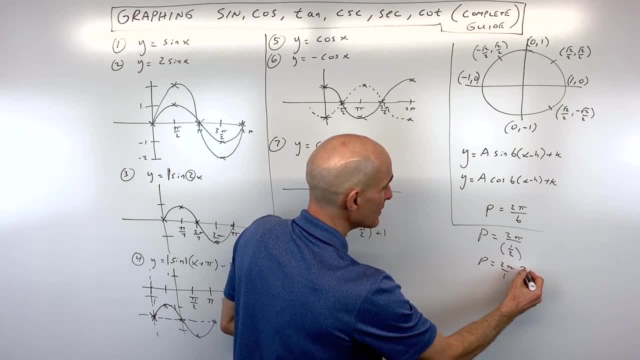 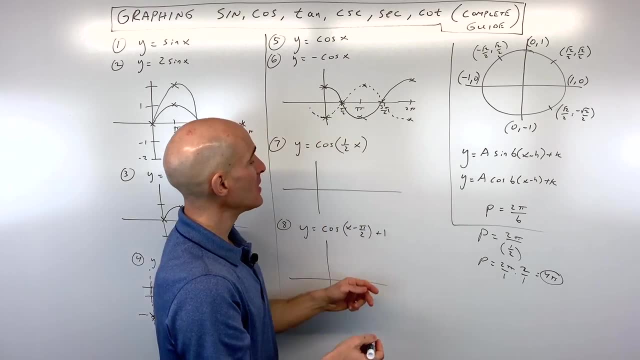 divide by a fraction, it's really like multiplying by the reciprocal. So, instead of dividing by one-half, 2 over 1, which gives us a period of 4pi. So what I like to do is I like to mark my x-axis with the. 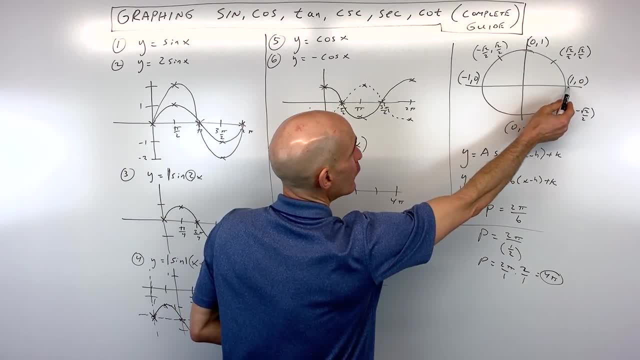 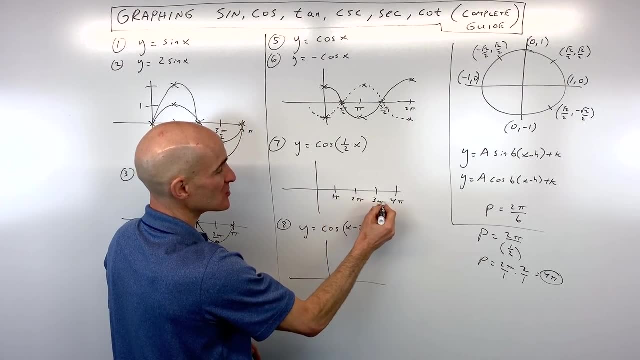 period 4pi, And I divide it up into four pieces, just like the four quadrants 1,, 2,, 3, 4.. So our scale is going to be pi, And then times 2 is 2pi, And then times 3 is 3pi, 4pi. So I just took 4pi. 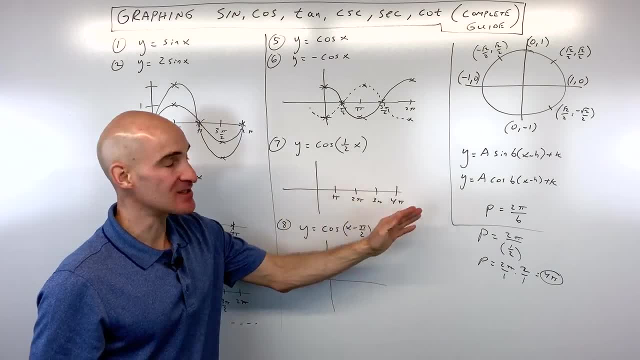 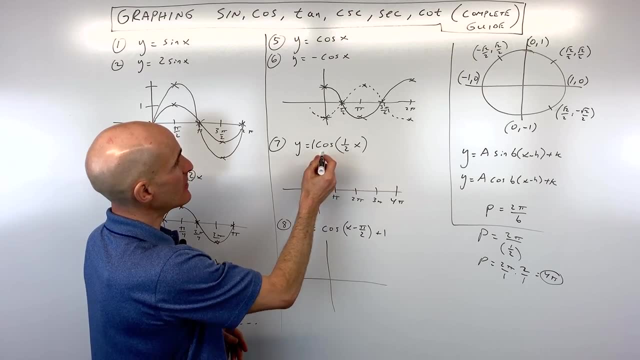 divided by 4.. And that's what I'm counting by to get to each successive point. on the x-axis, Our amplitude is 1, because 1 times anything is itself And we know cosine has that basic shape where it starts at the max And then it goes up to the max, And then it goes down to the max, And 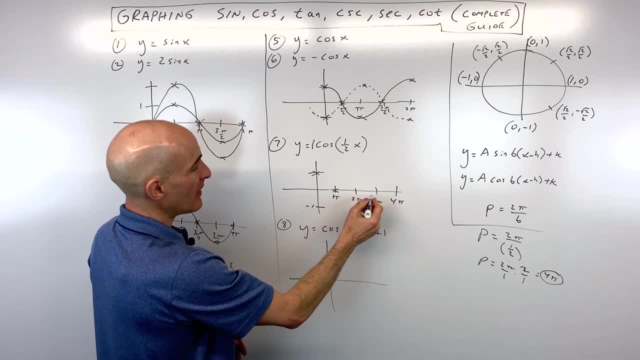 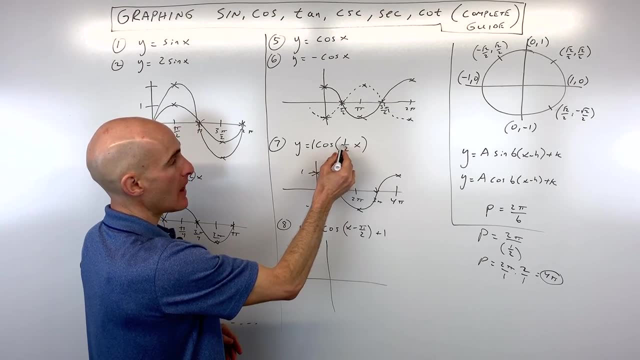 then it goes down to the maximum, back to the midline, down to the minimum, back to the midline, and then back to the maximum, And that's your basic graph. The only thing that changed here was, instead of dividing x's by 2, we actually did the opposite: We multiply the x's by 2.. That's why our 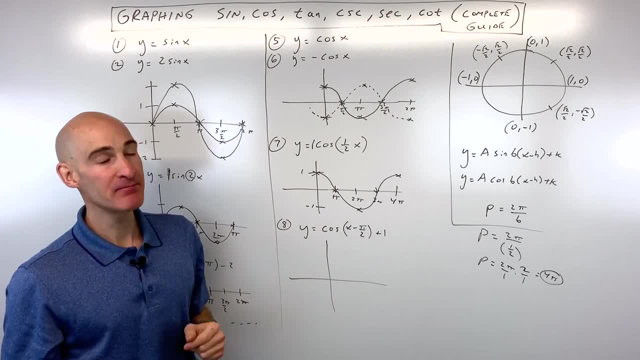 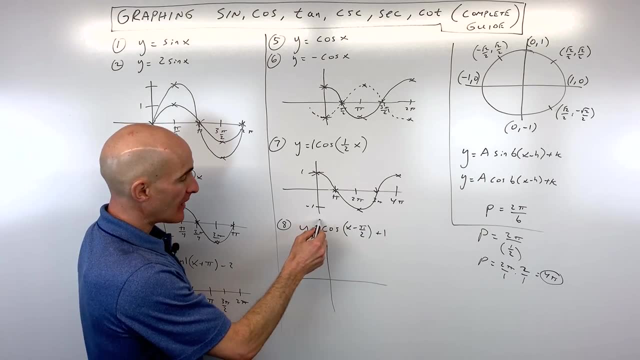 period is 4pi instead of the normal period of 2pi. So let's go to number 8. now We've got y equals cosine of x minus pi over 2 plus 1.. You can see the amplitude is 1.. The period is going to be the. 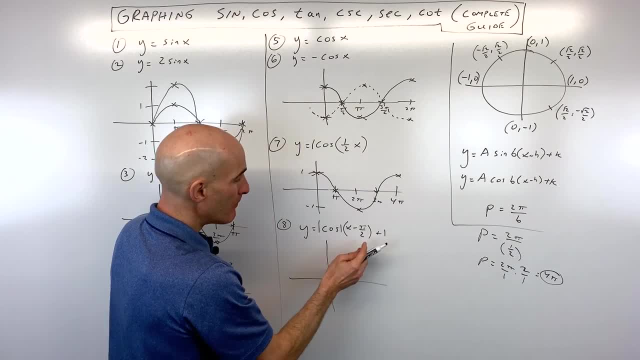 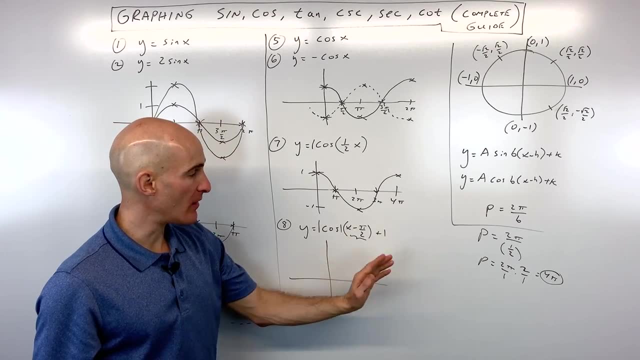 pi divided by the b value here is 1.. It's just going to be 2pi. But what's happening is the graph is shifting right: pi over 2.. Remember, the one group of the x has the opposite effect. Minus pi over 2, you're actually going right: pi over 2.. And then plus 1 is going to shift up 1.. So what? 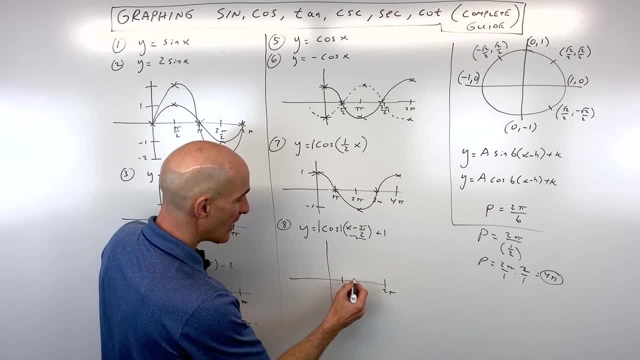 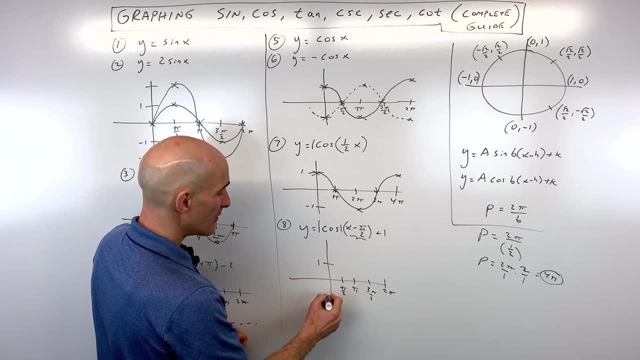 I'm going to do is I'm just going to label my x-axis 2pi, divide it up into four pieces. That's going to be pi over 2, pi, 3pi over 2, and 2pi. And we can see we haven't, it's not being stretched. 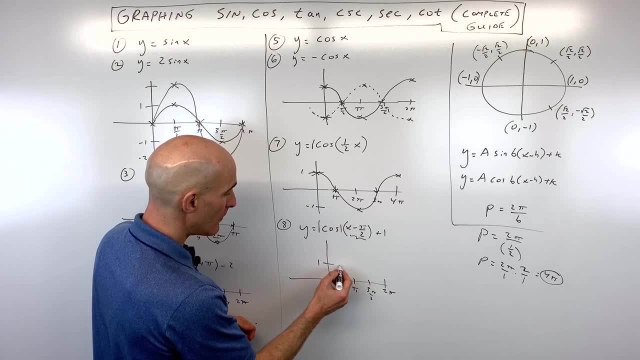 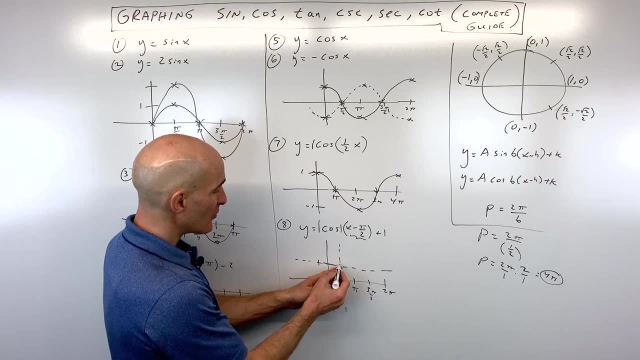 at all in the vertical direction. But what's happening is we're shifting right: pi over 2, up 1.. We can think of that as our new starting point or, like our new origin, It's a cosine graph. Remember, the cosine starts at the maximum. So you're going to start up here, You're going to 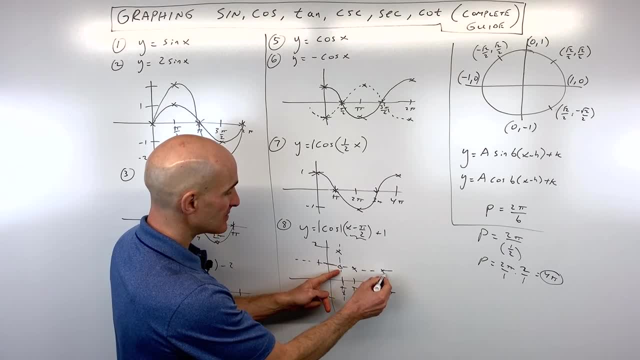 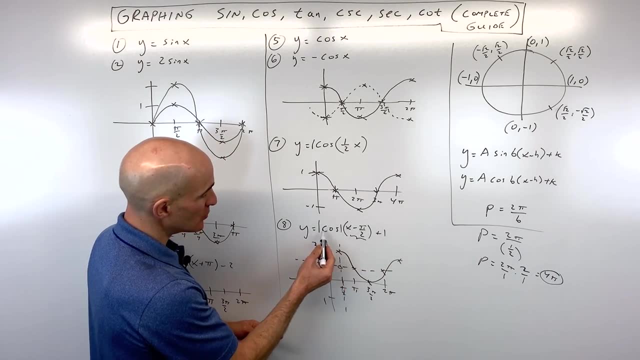 go back to the midline, down to the minimum, back to the midline and then back to the maximum. So that's your basic graph right there. Now notice the amplitude is 1.. So from that starting point, that's why I went up 1.. And then the minimum. I went down 1 from the midline. 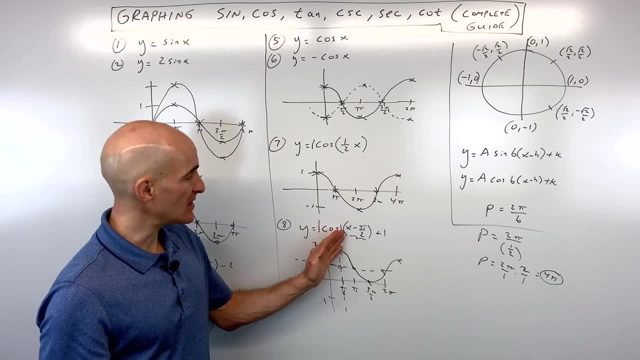 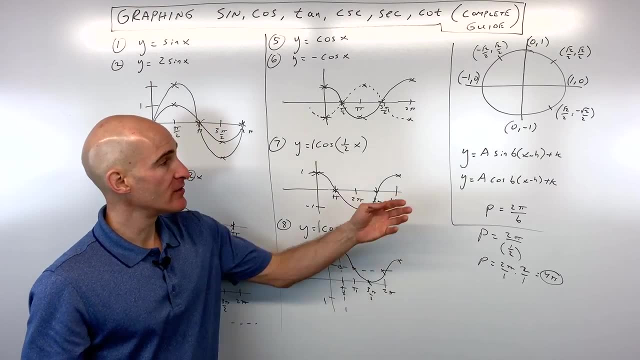 Again you have that basic shape. It had a normal period of 2pi. It was just everything was being shifted right: pi over, 2 and up 1.. Let me erase the whiteboard. I've got some more challenging problems involving all of the different components: a, b, h and k. Let's look at those next And then 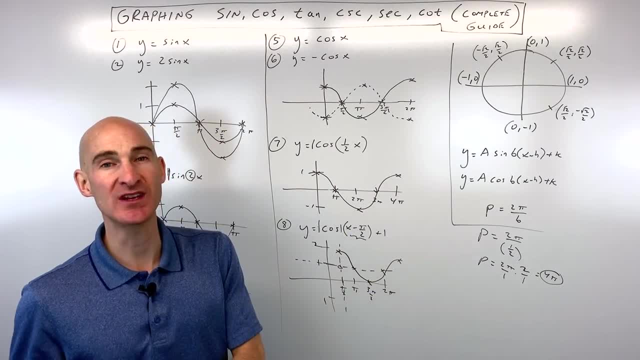 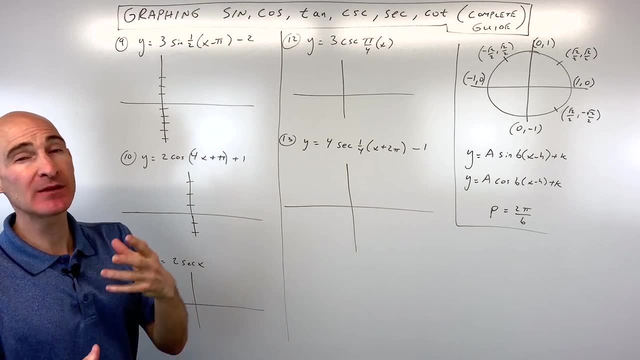 we'll jump into graphing the cosecant, the secant, and then the tangent and the cotangent. Okay, number 9.. Let's look at: y equals 3 sine of 1, half x minus pi minus 2.. So we've got a little bit of. 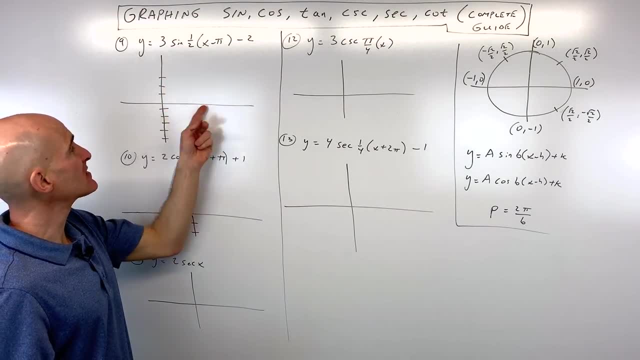 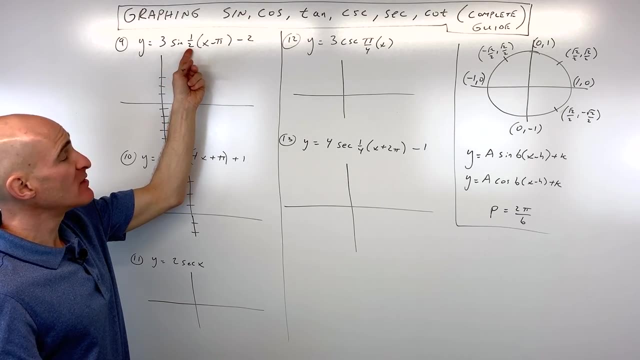 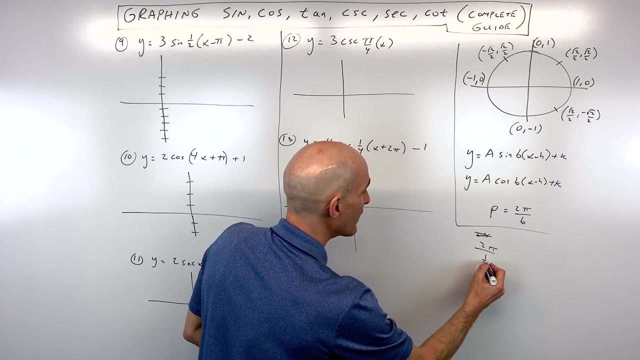 everything in this problem. The first thing I like to do, though, is I like to look at the scale on the axis, the horizontal stretch, or compress, So let's figure out what the period is. We've got the b value of 1 half, So 2pi divided by 1 half looks like. let's see. so 2pi divided by 1 half, We know. 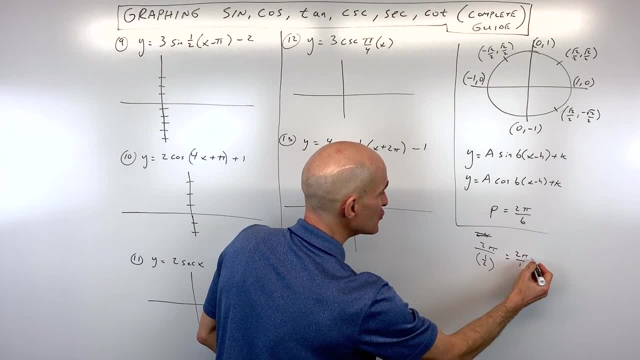 when we divide by a fraction, it's like multiplying by the reciprocal, So that's going to be like 2pi times 2 over 1, which is 4pi. So we're going to go ahead and mark our scale. We've got 4pi Divide. 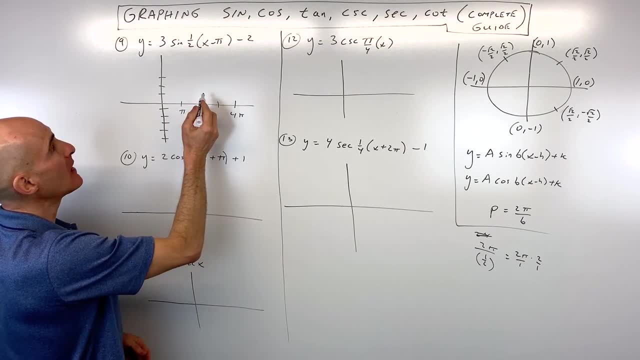 that by 4.. We get 1pi, 2pi, 3pi, 4pi, But you can see that the graph is shifting left pi, I'm sorry, minus pi is actually having the opposite effect. It's shifting right pi and then down 2.. 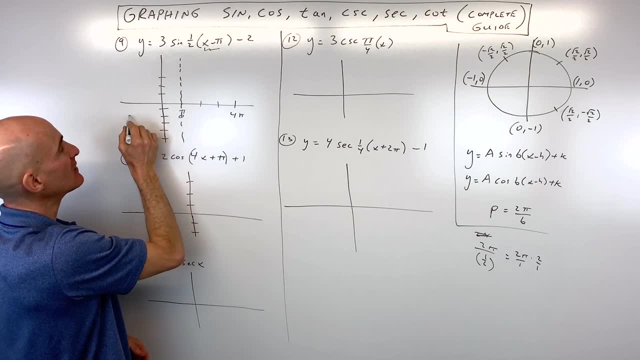 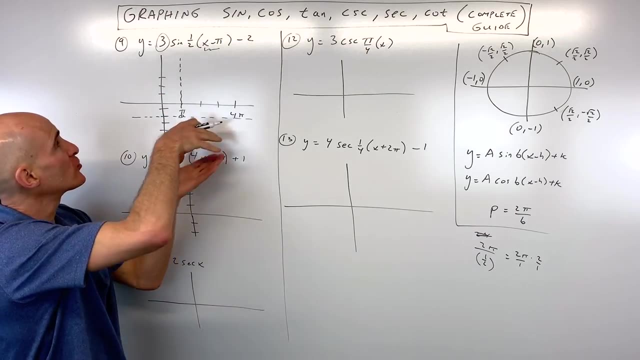 So we can think of this as our new starting point, right pi down 2.. And that's your point right there. Now you can see the amplitude is 3.. So that's a vertical stretch of 3.. And we know we 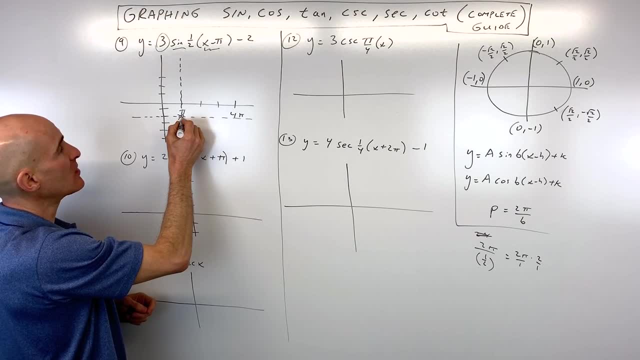 have a sine graph. So we can see that from this point it's going to start here. It's going to go up 3.. So let's see, when you're over here you're going to go up 3,, 1,, 2,, 3.. That's the maximum. 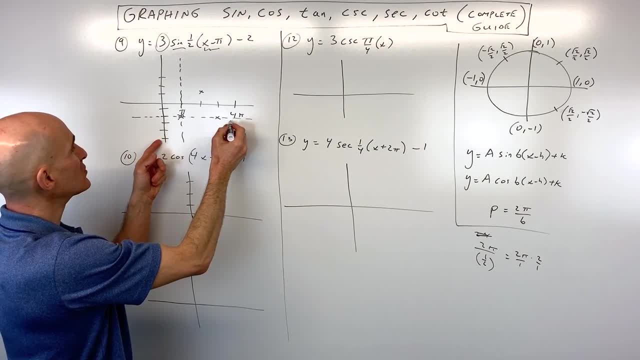 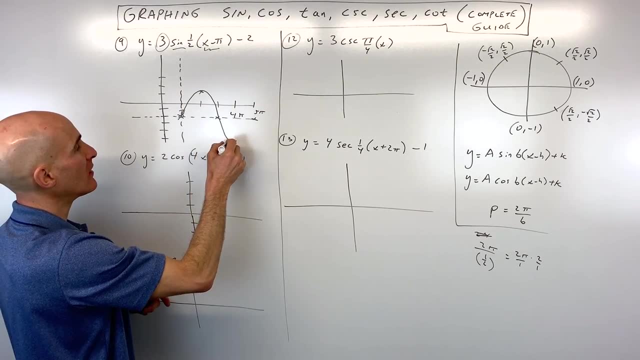 Back to the midline, Then down to the minimum- 1,, 2,, 3, which is going to be right down here, And then back to the midline And you've got one period of your sine graph Again. notice that the one that's grouped- 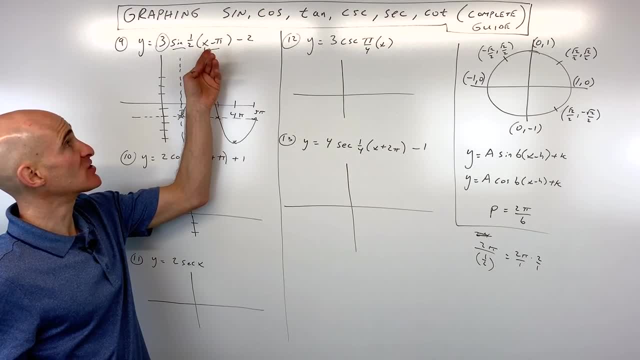 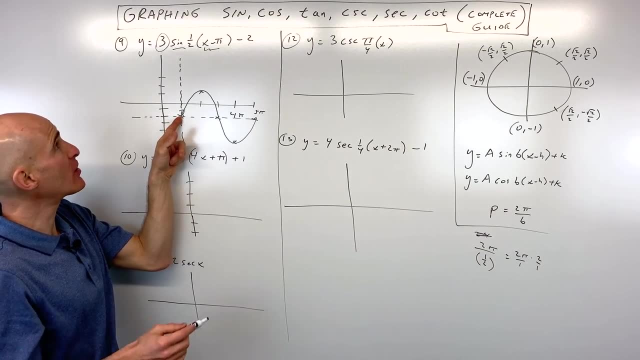 with the x. that's going to be the phase shift. It's going to have the opposite effect. Minus pi shifts right pi- This is your vertical shift, your k value shifting down 2. Think of that as your starting point. Pay attention to whether it's a sine graph or a cosine graph, And then 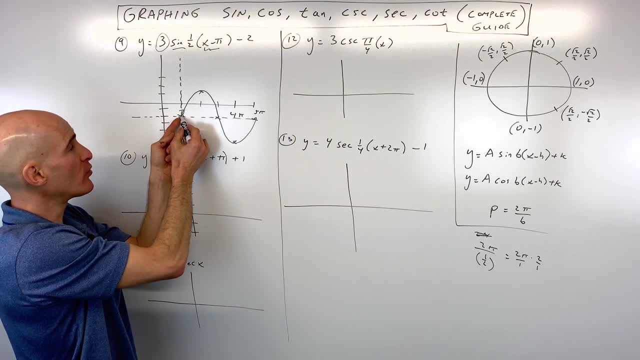 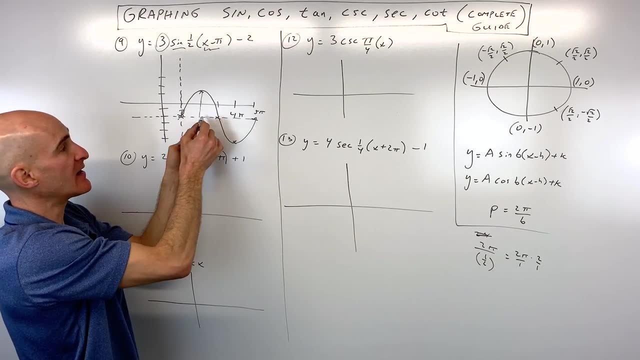 the amplitude is a vertical stretch, So think of it as your new starting point. Sine starts at that origin, goes up to the maximum, But that maximum is going to be 3 units from that midline. Same thing with the minimum It's going. 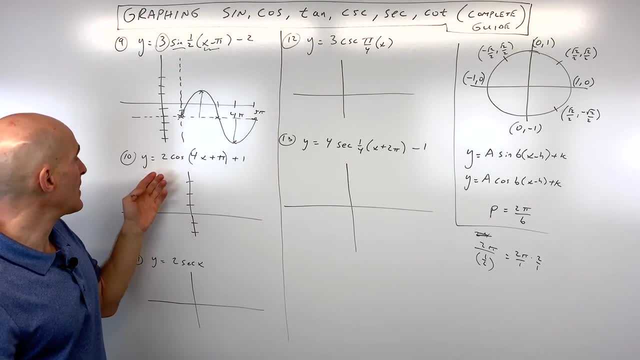 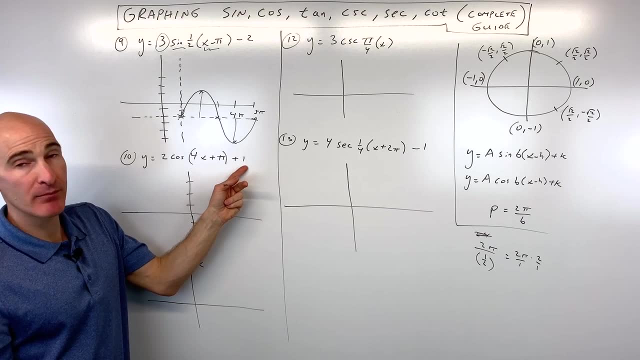 to be 3 units from the midline, And you've got it. So let's look at another example involving all the different components here. Number 10, y equals 2 times cosine of the quantity 4x plus pi plus 1.. 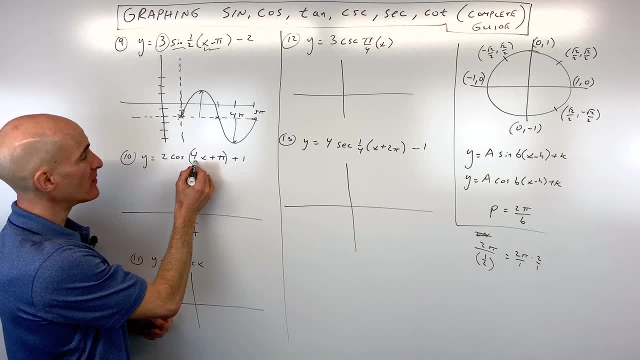 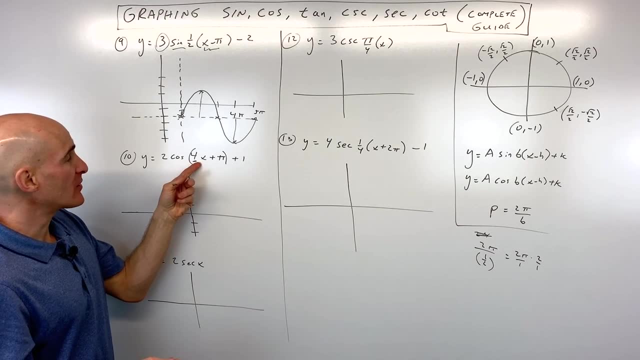 Now, what's different about this problem is see how there's a 4.. Okay, this b value. it's inside of the parentheses. It's grouped with the x. What we need to do is we need to group the x with the y, We need to factor it out. And when you factor the 4 out, you're going to have to factor it out of. 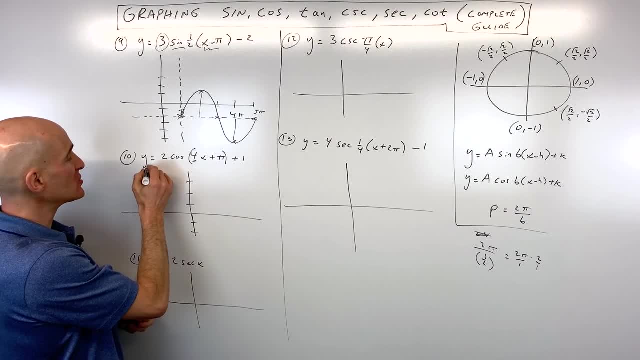 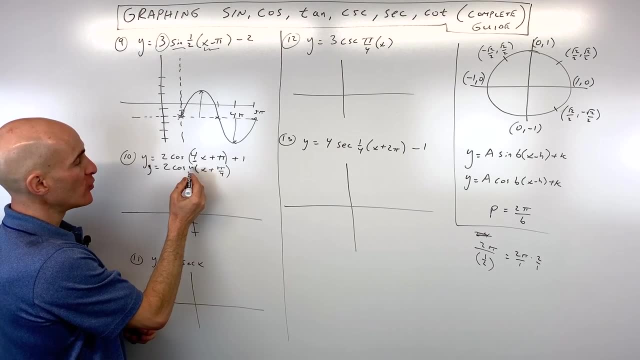 both of these terms. So we're dividing out 4.. So our equation is going to look like this now: y equals 2 times cosine of 4x plus pi over 4.. Notice, if you distribute that 4 back in, you get 4x plus. 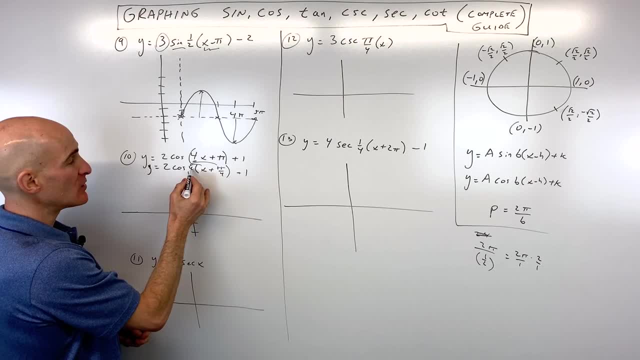 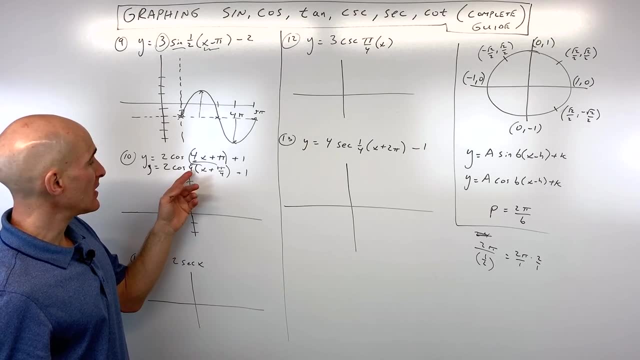 4pi over 4,, which is 1pi. So that's the key. You definitely want to have just 1x inside of the parentheses, So you have to factor out that coefficient So you can see here that the b value. 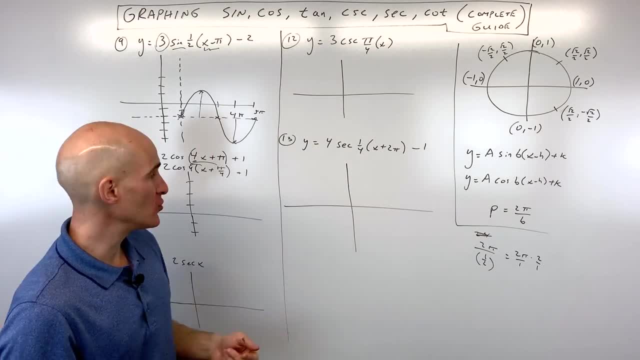 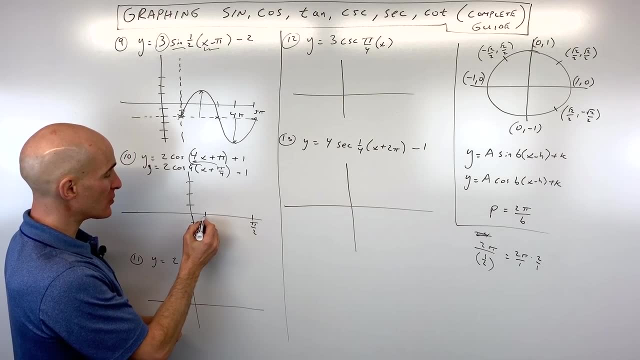 is 2pi over 4.. So if we take 2pi divided by 4, that reduces to pi over 2.. So that's our period: pi over 2.. If we divide that by 4 or multiply it by 1 fourth, either way you're going to get pi. 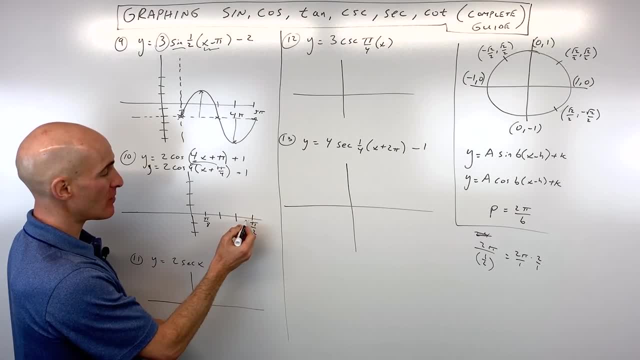 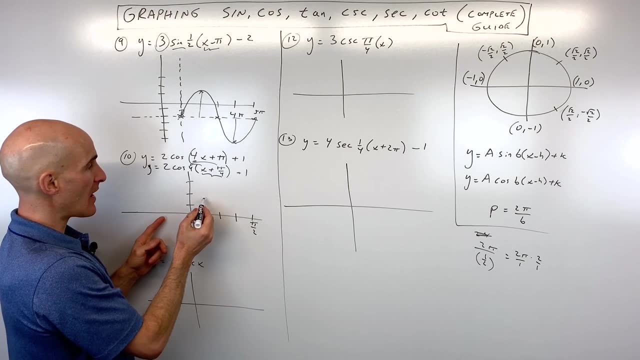 over 8.. That's our scale, So 1pi over 8,, 2pi over 8, 3pi over 8, 4pi over 8.. We can see that our graph is shifting left pi over 4, because, remember, this has the opposite effect on the graph. So it's: 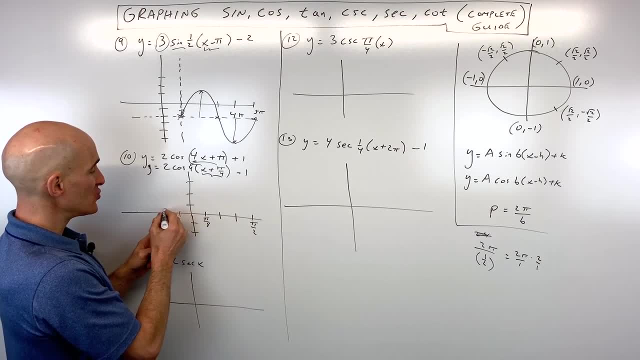 going to go left pi over 4.. So pi over 4 is actually two steps. So left pi over 4, because pi over 8 times 2 is 2pi over 8, which is pi over 4.. So we're going to get 2pi over 8,, 2pi over 8,. 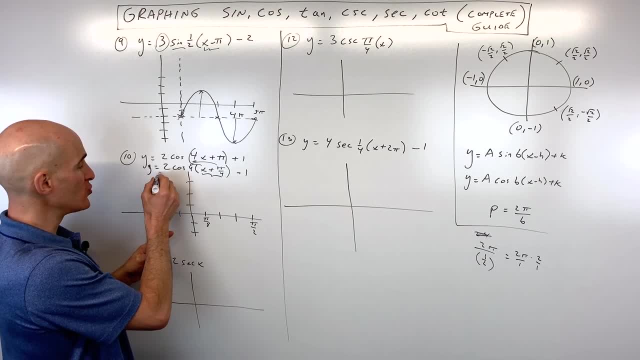 2pi over 4.. And then plus 1 is going to shift up 1.. So that's our new starting point. We can think of that as our new y-axis, our new x-axis, our new origin. It's a cosine graph with an. 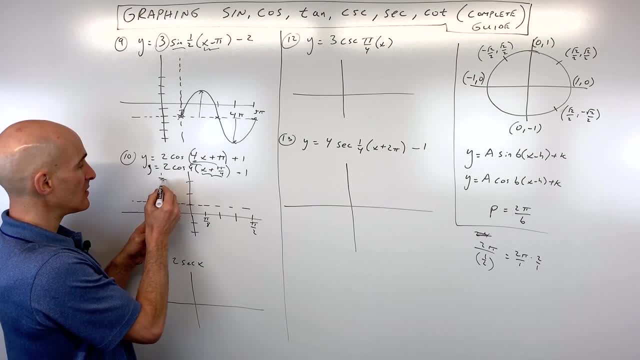 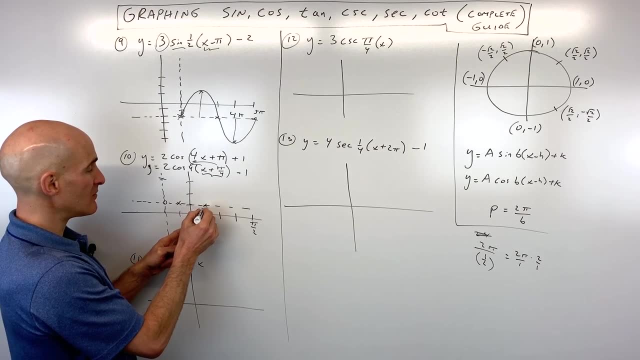 amplitude of 2.. So from here it's going to start at the maximum, So I'm going up 2, back to the midline, down to the minimum, So that's going to be down 2, back to the midline and then back to. 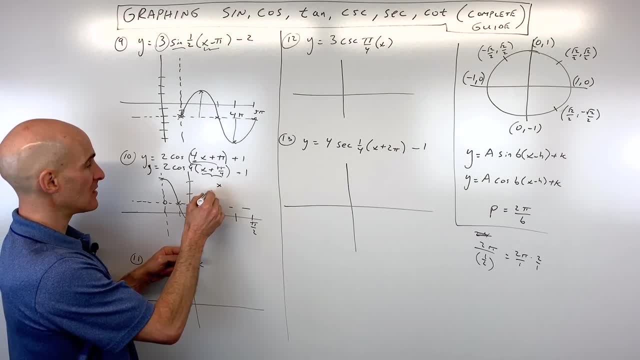 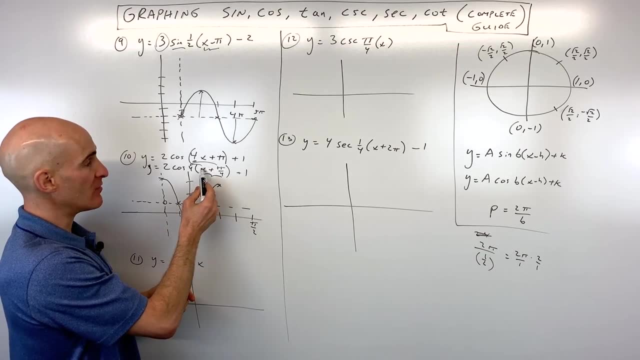 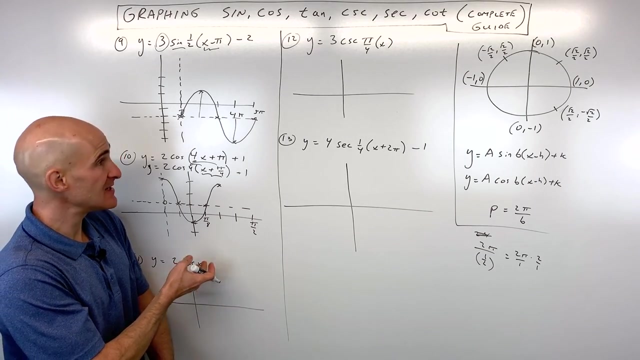 the maximum up 2.. So that's going to be our basic cosine shape. The only difference is that it's also being shifted and the period is changing as well. So that was a good example. So now what we're going to do is we're going to transition over to working with the secant and the cosecant. 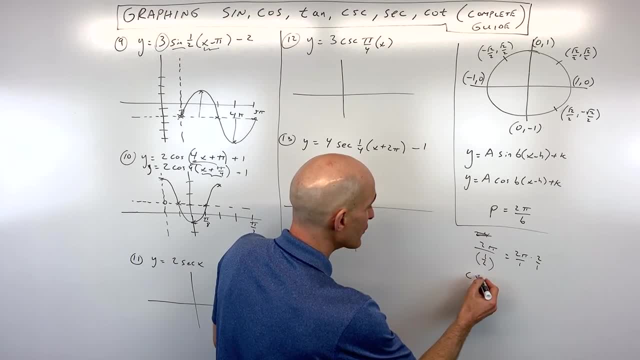 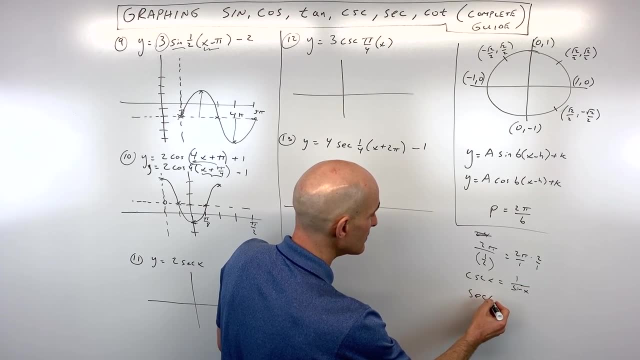 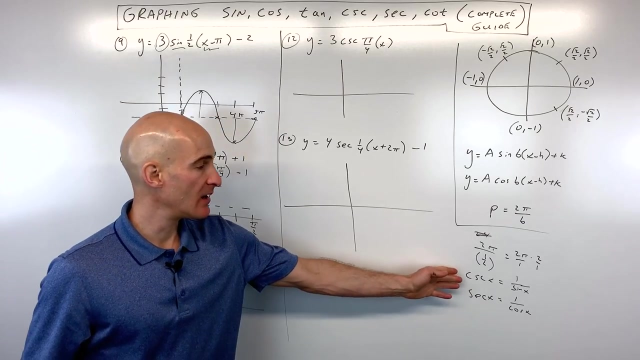 graphs. So just a quick refresher: When you think about the cosecant, it's really the reciprocal of the sine graph see 1 over sine. And when you think of the secant function, it's the reciprocal of the cosine function, so 1 over cosine. So we're going to use that information to graph these. 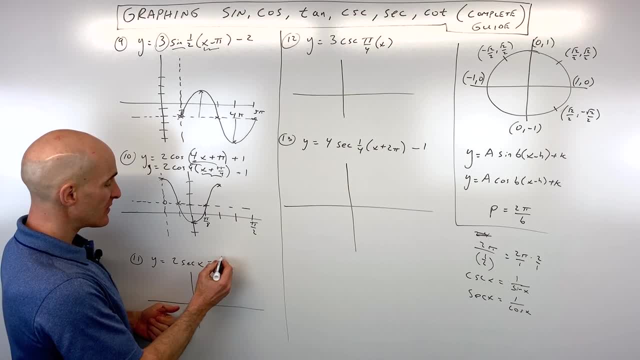 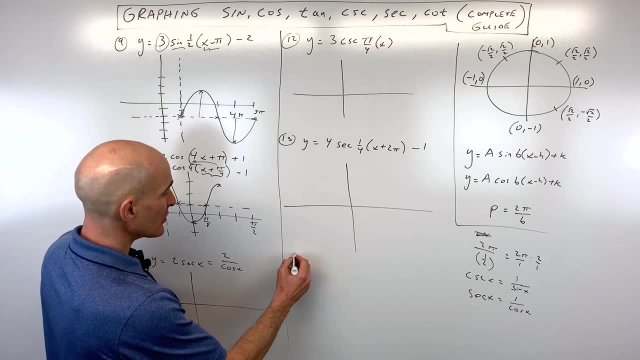 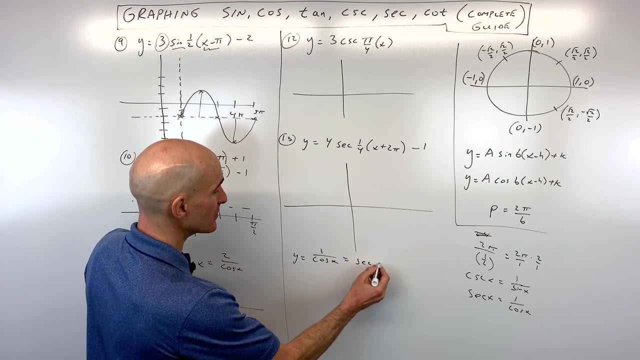 graphs. So when we look at y equals 2 secant of x, we can think of this as 2 over cosine of x. Now let's start a little bit simpler. Let's just say we wanted to graph: y equals not cosine of x, but 1 over cosine of x, which is equal to secant of x. So let's look at our basic. 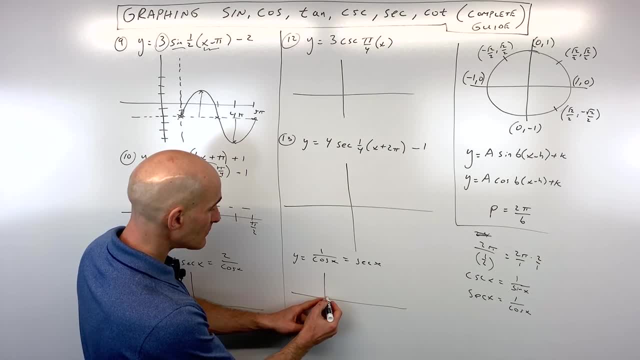 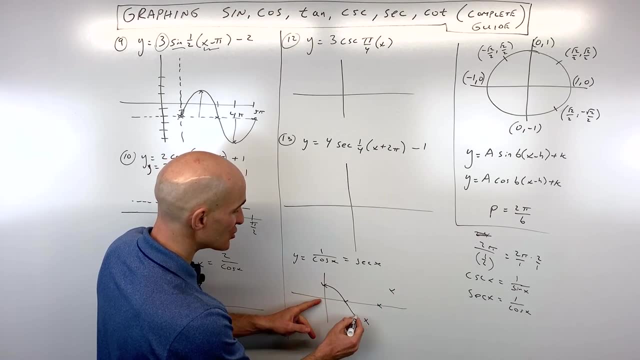 values on the unit circle. So when we think of cosine, we said cosine starts at the maximum, it goes to the midline, then to the minimum, then to the midline, back to the maximum. That's the basic shape, right? This is 1,. this is negative 1, this is pi. 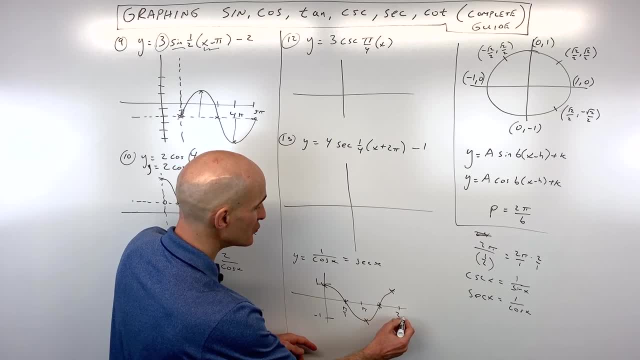 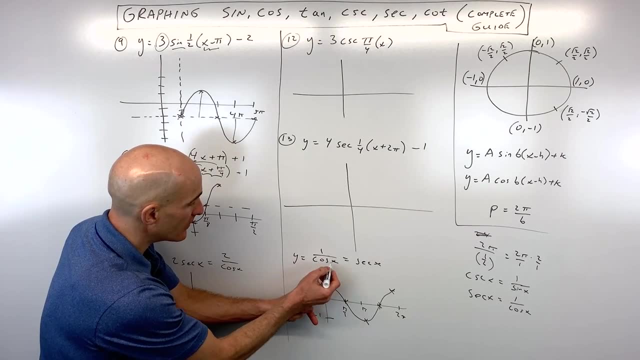 over 2, pi, 3 pi over 2, and 2 pi. right. But here's the thing: When you're at 0, see how the cosine value is 1? So if this is equal to 1, right here. 1 divided by 1 is still 1, right When you're. 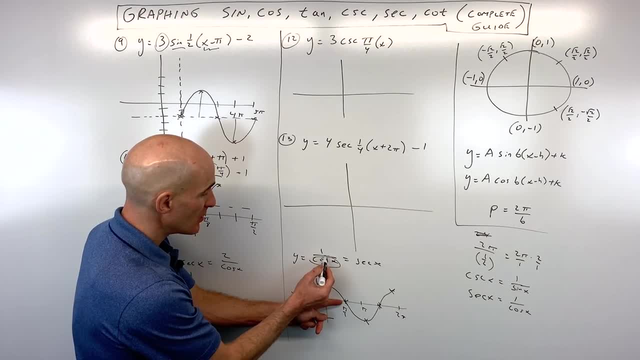 over here at 0, pi over 2, see, this is 0, what's 1 divided by 0?? Well, that's undefined. You can't divide by 0. So what happens is we get a vertical asymptote. So what happens is we get a vertical. 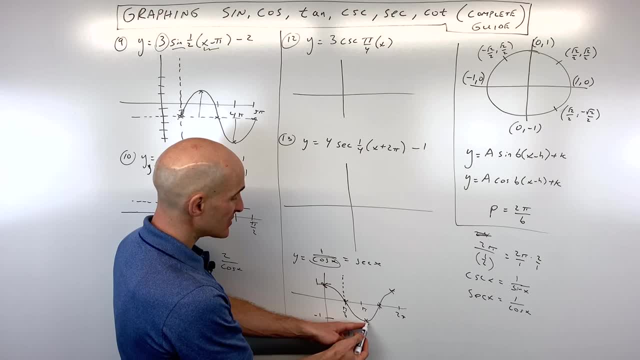 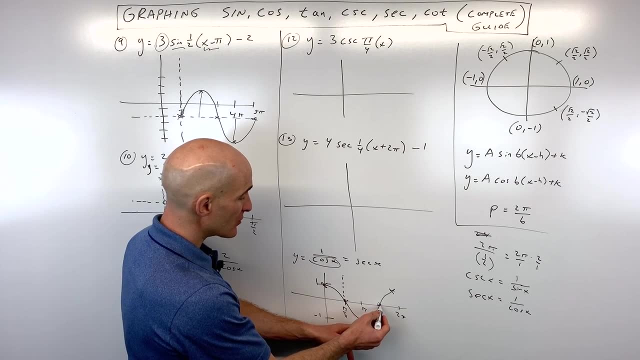 asymptote here: When you're at pi, cosine is equal to negative 1.. What's 1 divided by negative 1?? That's still negative 1.. And then, when you're over here at 3, pi over 2, that's 0. Again. 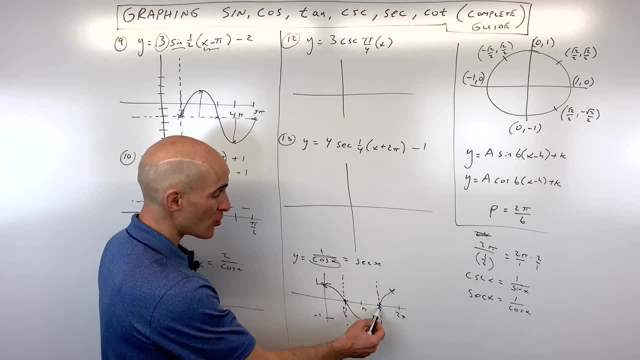 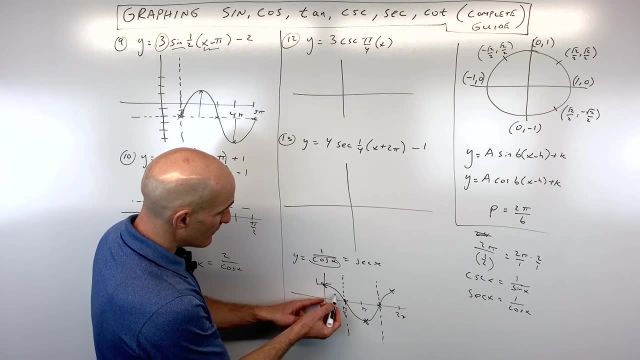 1 divided by 0 is undefined, You get another vertical asymptote. So wherever the graph is crossing the x-axis, that's where your vertical asymptotes are going to be. Now notice when I'm at this point. say, for example, right here, Say for example: this is like a cosine value of 1. 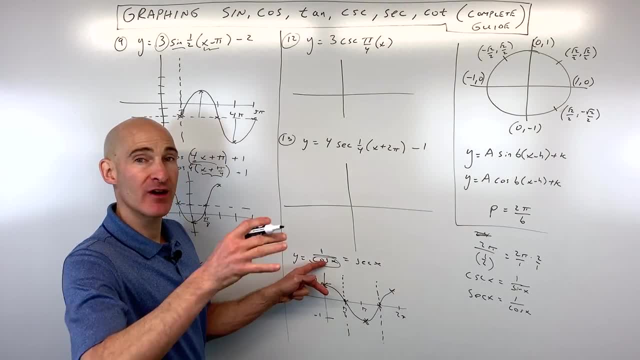 half. Well, 1 divided by 1 half. when you divide by a fraction, it's like multiplying by the vertical. So 1 divided by 1 half is really going to be like 2.. You're up here So you can see this. 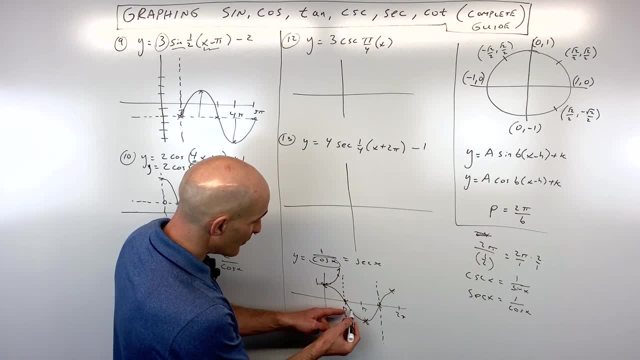 graph is looking like this. now, When you're over here, let's say like when cosine is negative 1, half, 1 divided by negative 1 half is going to be like negative 2, right. So this graph is looking something like this, et cetera. So what you can see is the cosine graph. if you graph that, 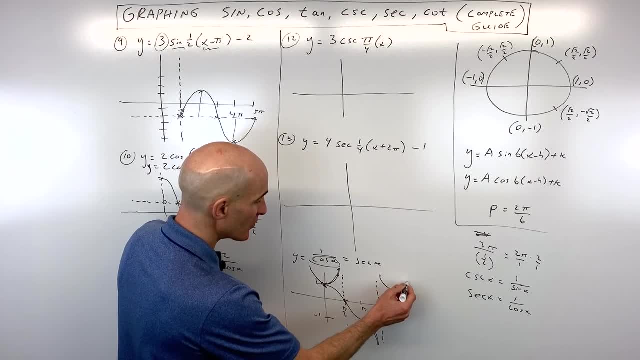 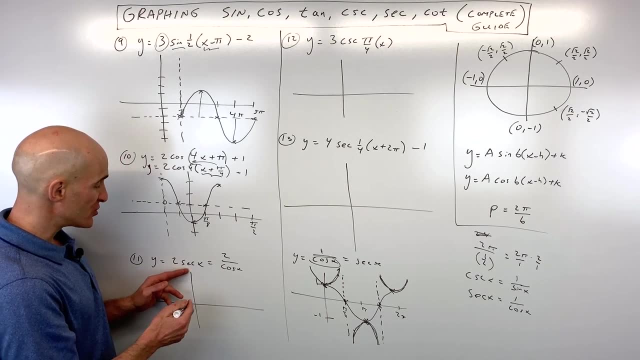 and you look at these key points, where it reaches a maximum or a minimum, that's going to be where the secant graph bends or turns. Okay, so I'll show you another example. So say for example this one: y equals 2 secant of x. What you would do is you would start by graphing: y equals 2. 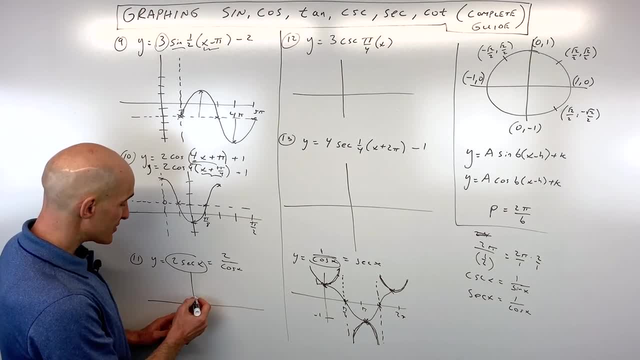 cosine of x. So cosine of x looks like this: It has an amplitude of 2.. Okay, it has a period of 2 pi, like that, Wherever it crosses the x-axis. those are where our asymptotes are going to be. 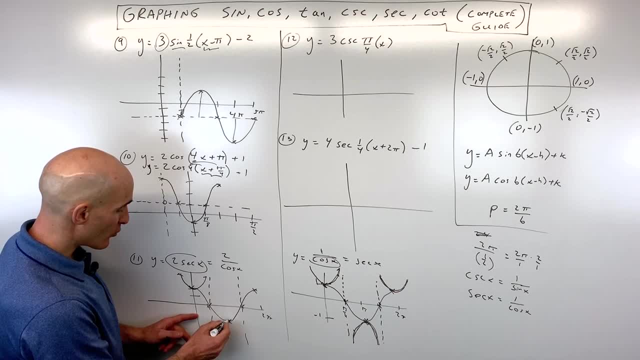 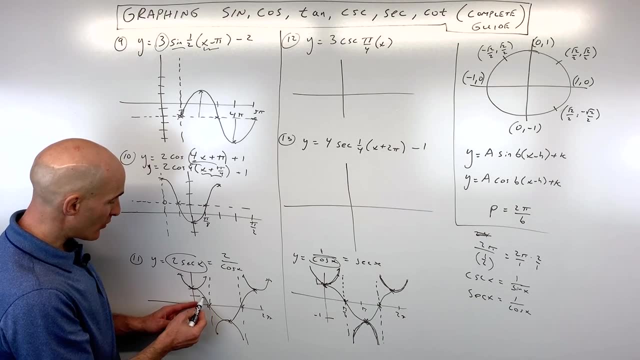 And then the secant graph is going to have the shape where it goes the opposite direction, like that. Okay, And again, the reason it works is because, see how, when this value is, let's say, for example, 1,. 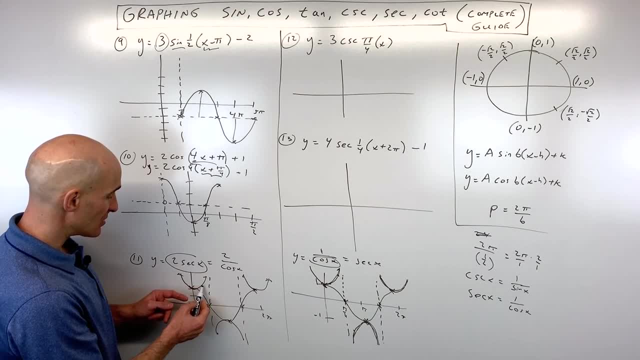 well then you have 2 divided by 1, which is actually going to be 2, right? And then same thing over here, When this is like a half 2 divided by 1, half, that's going to be 4.. So you, 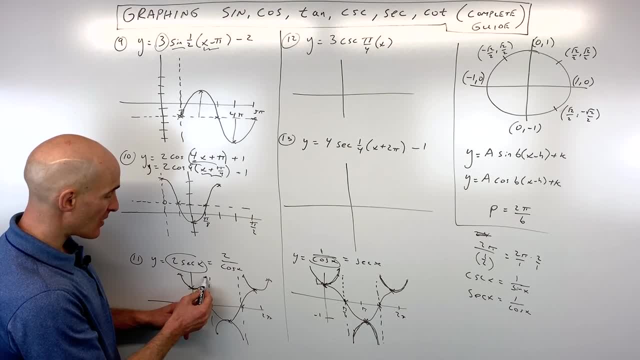 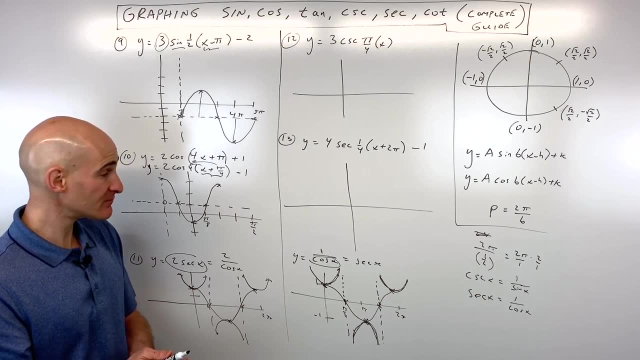 can see that as this gets smaller and smaller- the cosine graph, the secant graph- it's going to be larger and larger, Because when you divide by a smaller and smaller fraction, you're multiplying by the reciprocal. this is going to go up and up and up. So that's the same idea when you're 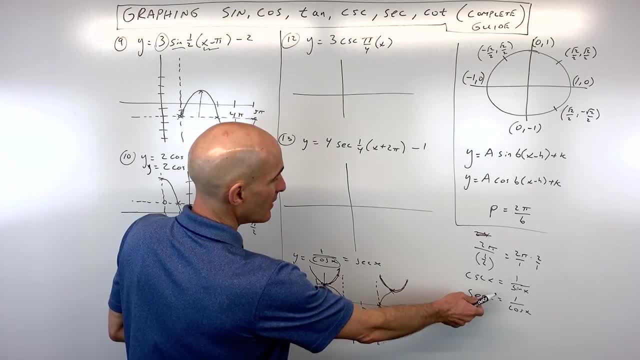 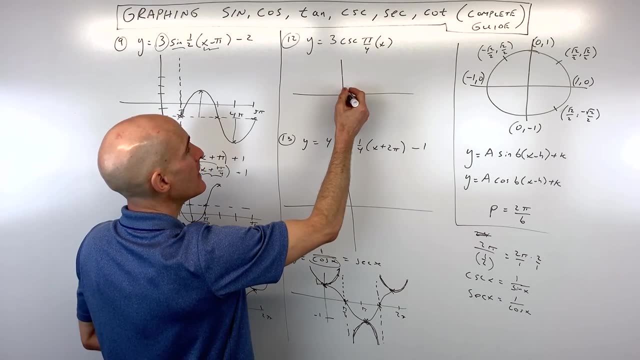 working with the cosecant graph. Remember, secant is the reciprocal of sine. So if we wanted to graph this graph, let's just graph: y equals 3 sine of pi over 4 times x. The sine graph we know looks like this: Okay, The amplitude is 3.. 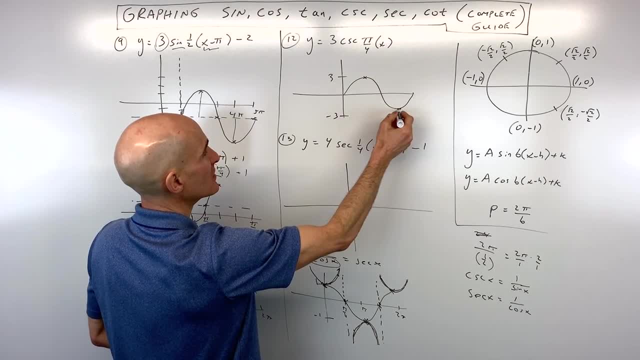 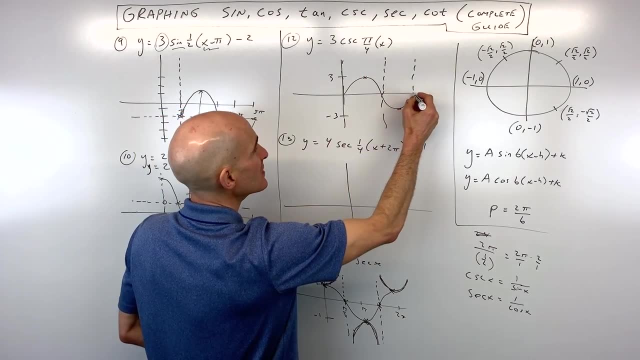 So it's going to reach a maximum here at negative 3 and on positive 3 and down to negative 3.. Wherever it crosses the x-axis, that's where our vertical asymptotes are Okay. Sometimes, when you're doing the secant and cosecant graphs, it helps to draw, you know, a little bit more cycles. 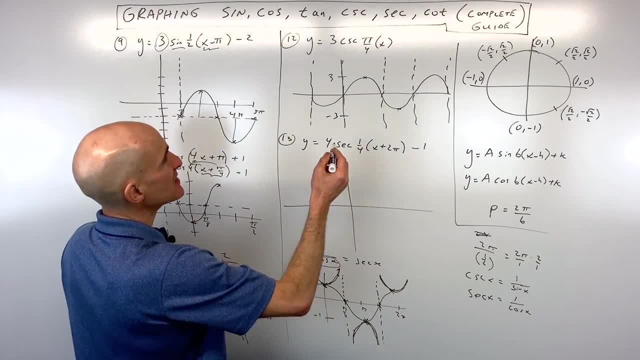 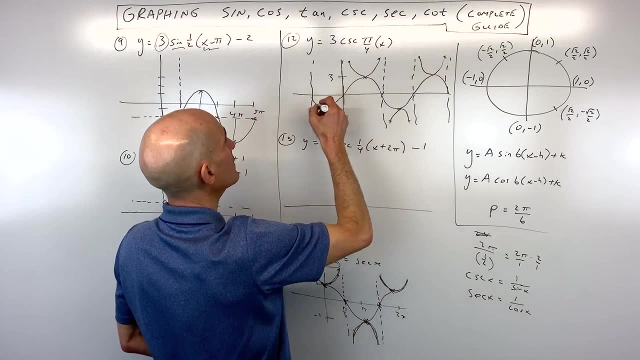 Okay, More periods. And then what you can do now is you can say our graph is going to look like this. Now, the one thing that I haven't done yet is look at the periods. Let me do that on last here. Usually I do it before I graph this, but I would take the pi over 4.. Remember, the period is 2 pi. 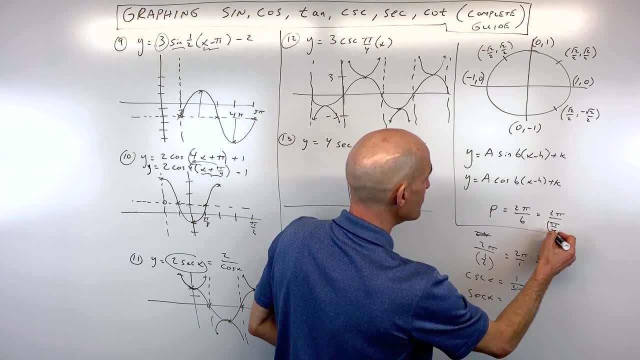 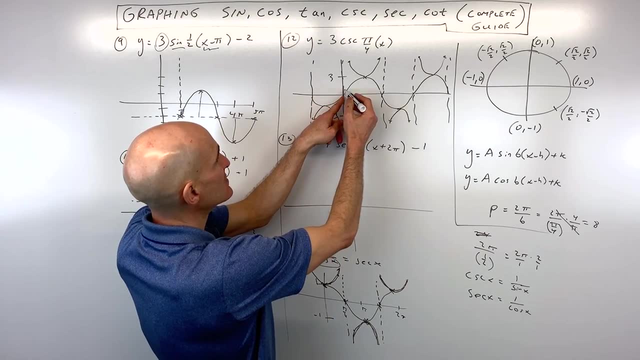 divided by pi over 4.. Okay, 2 pi divided by b, which is like multiplying by the reciprocal. So the pi's cancel and it's actually going to have a period of 8.. So you can see this is going to be. 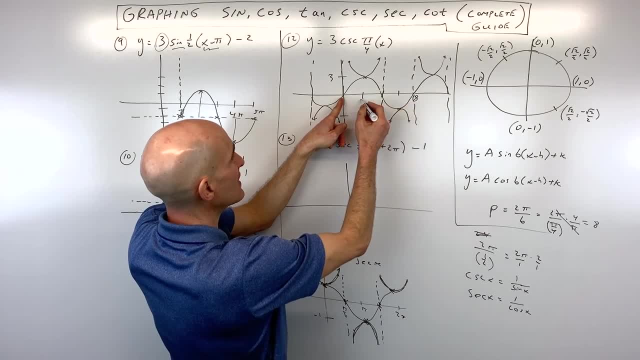 right here. This is going to be 8 divided up into 4.. So that's going to be 2 pi over 4.. So that's 4 pieces: 2, 4, 6, 8.. That's our scale And you've got your cosecant graph. Okay, Let's do a. 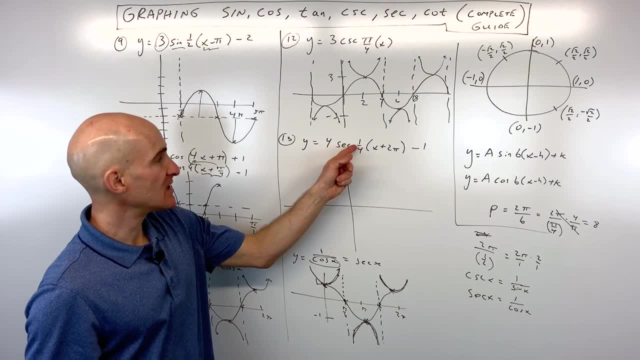 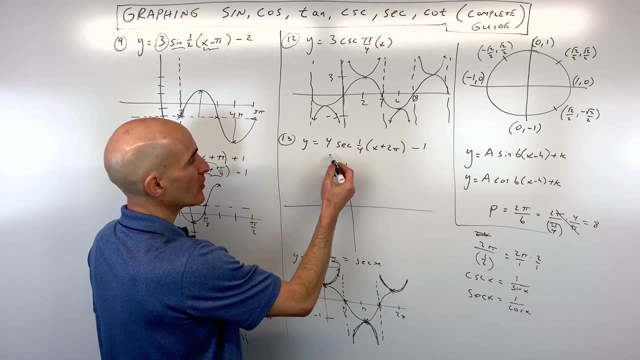 little bit more challenging one, Number 13,. we've got y equals 4, secant 1, 4th, x plus 2, pi minus 1.. So that's a lot right, But what we're going to do first is we're going to graph the same equation. 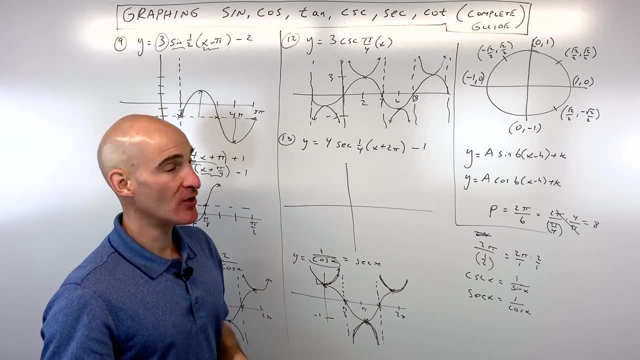 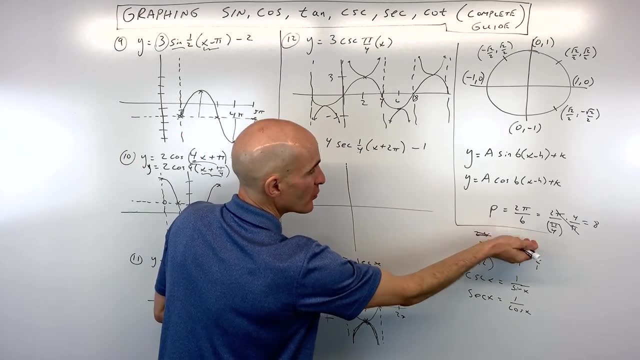 here, except for, instead of secant, we're going to think of it as cosine. Okay, If we take the period 2 pi divided by b, which is 2 pi divided by 1 4th, When you divide by 1 4th it's like: 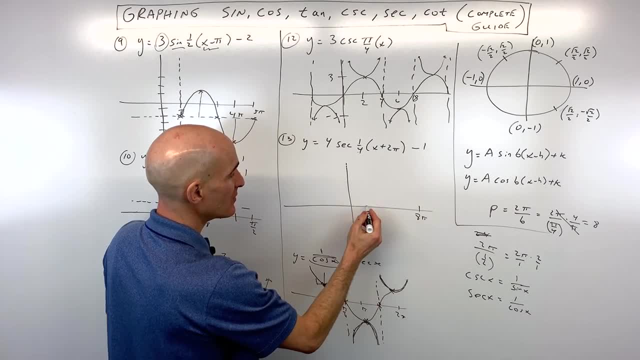 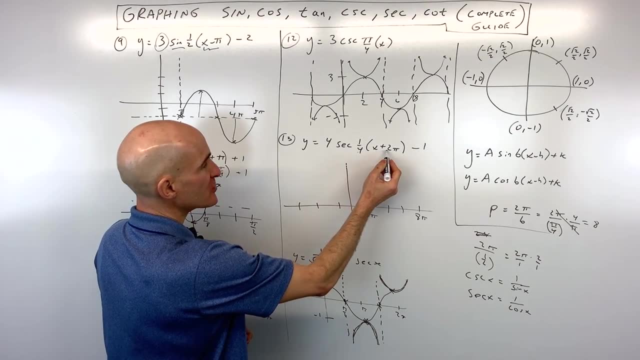 reciprocal, That's going to be 8 pi. So our period is going to be 8 pi here. Divide it into 4 pieces, That's going to be 2 pi, 4 pi, 6 pi, 8 pi. Okay, But the graph is shifting left, 2 pi down. 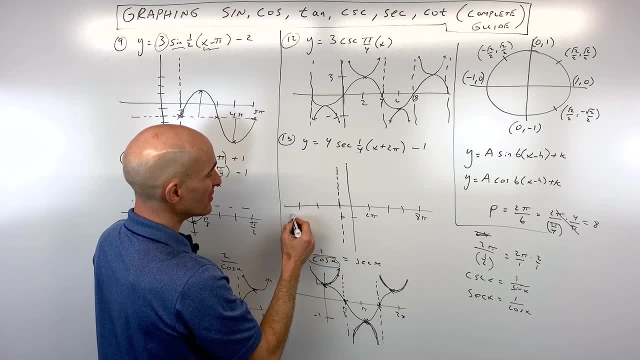 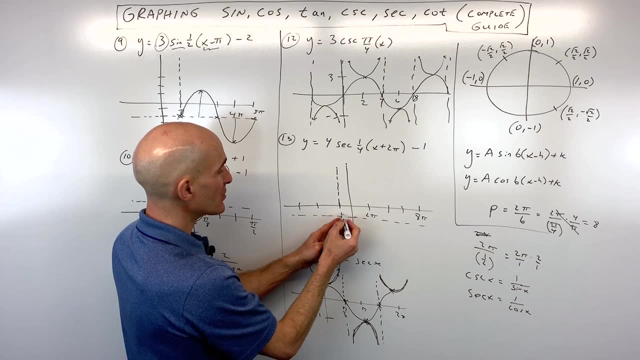 1. So we're going to think of this as like our new origin, like right, like that. Okay, And the amplitude is 4.. It's a cosine graph, So we're going to go up 4.. So this is going to be 1,, 2,. 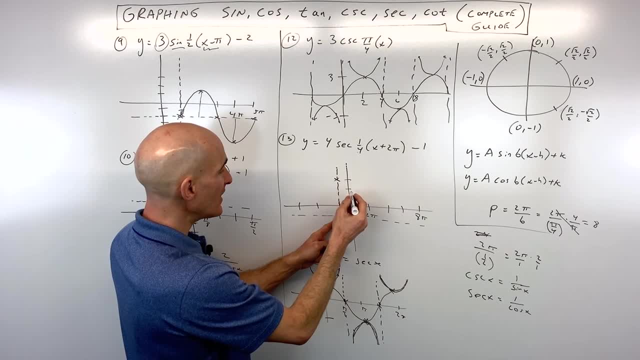 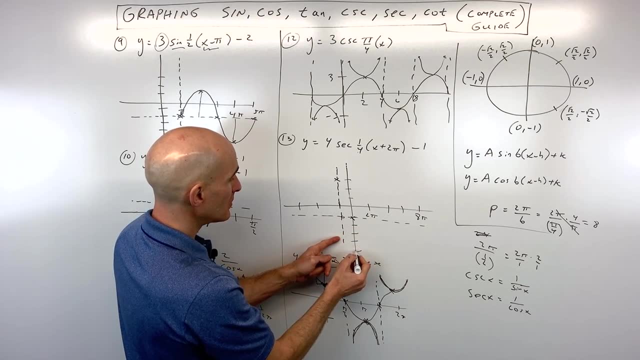 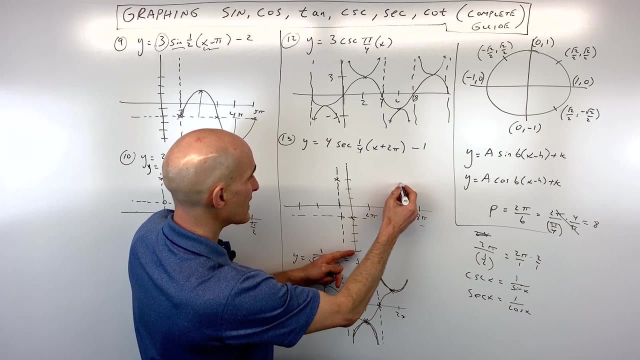 3, 4.. So it's going to start right here, It's going to go back down To the midline, Okay, And then it's going to go down to the minimum, which is going to be right here at down: 4 from the midline, then back to the midline and then back to the maximum, Okay. 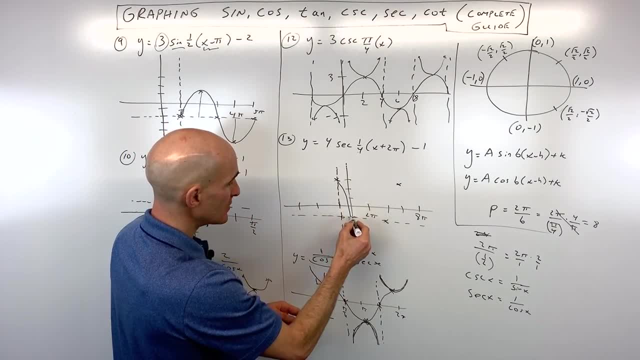 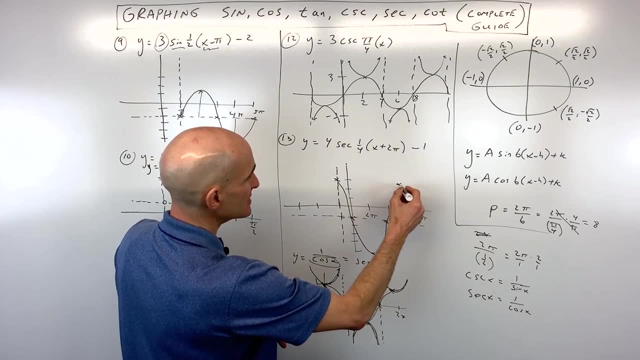 Which is 4 above the midline, because the amplitude here is 4.. So that's going to be your basic. Let's see your basic graph, something like that. Okay, And it's going to continue. Okay. But what we need to pay attention to is where this cosine graph crosses the 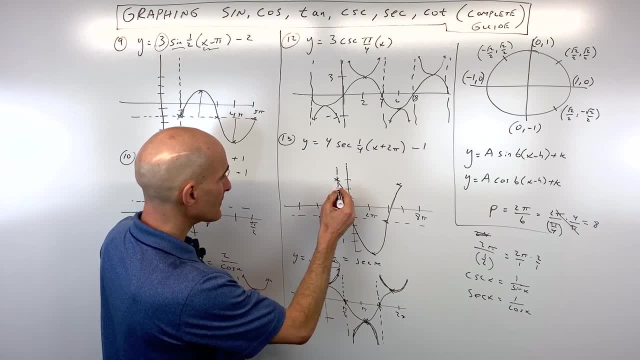 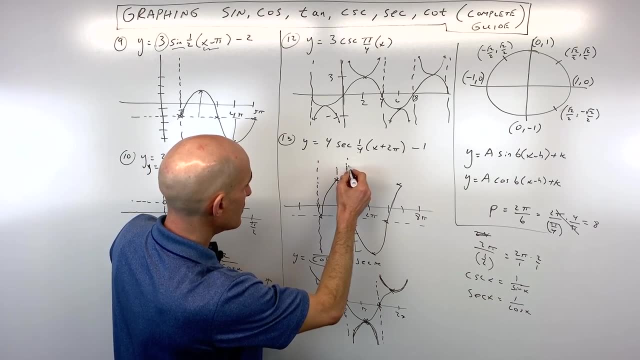 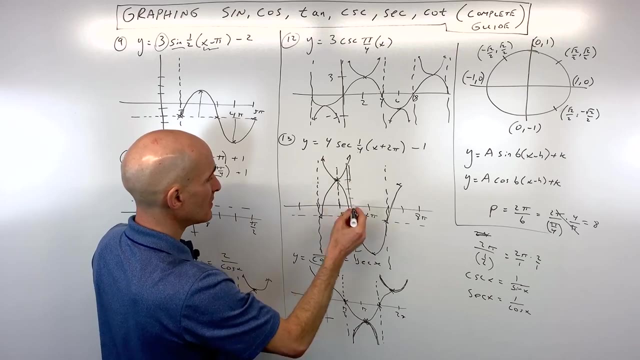 midline, Okay, So it's crossing, basically like this: So it's crossing right here, It's crossing right here, Okay, It's crossing right here, et cetera. So our secant graph is actually going to look like this: It's going to approach the asymptotes, but it's not going to cross them, or. 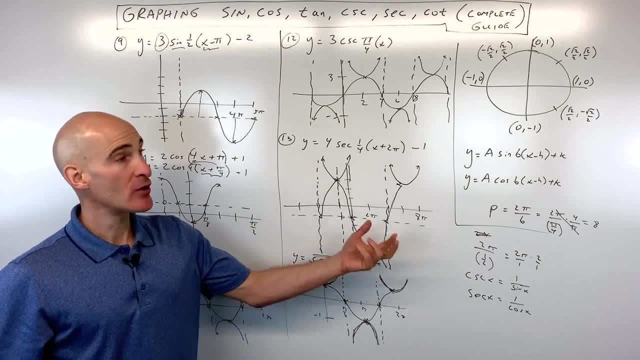 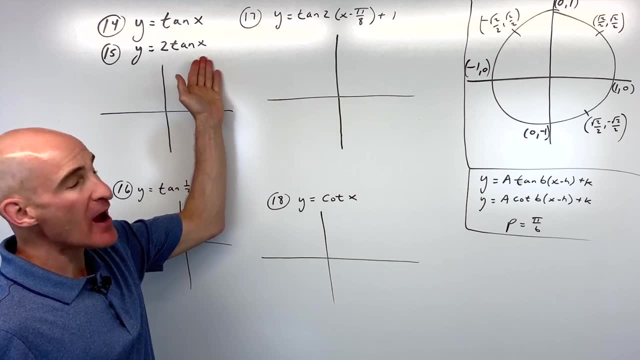 touch them. So that's the basic idea, and you've got it. So let me erase the whiteboard. We're going to talk about tangent and cotangent next. Okay, Now, switching gears over to tangent and cotangent. When you graph tangent, we're going to be using 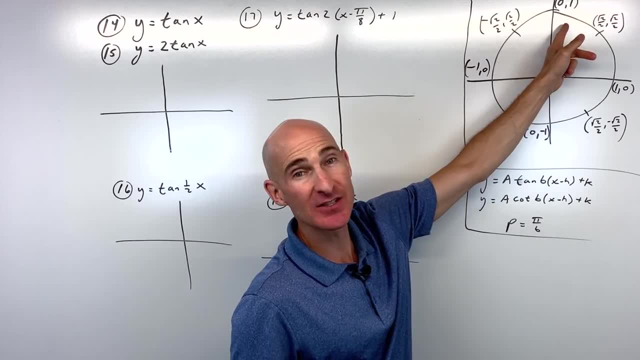 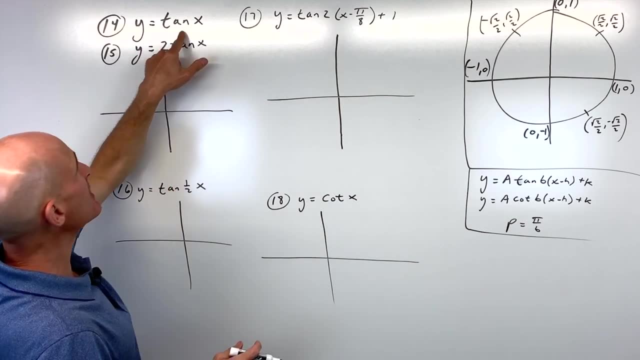 the values from negative pi over 2 to positive pi over 2.. And remember from the unit circle the tangent's, the y value divided by the x value. So let's just go ahead and graph the basic parent graph first, And what I'm going to do is I'm going to start over here at negative pi over 2. 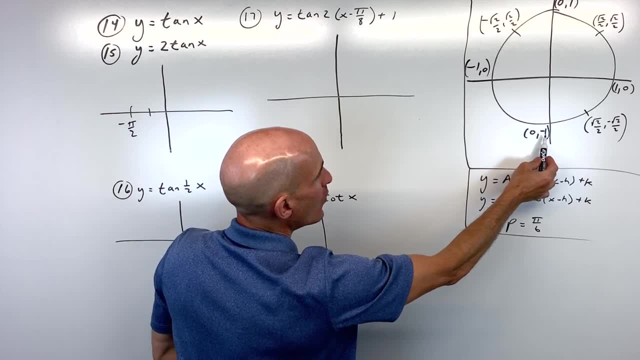 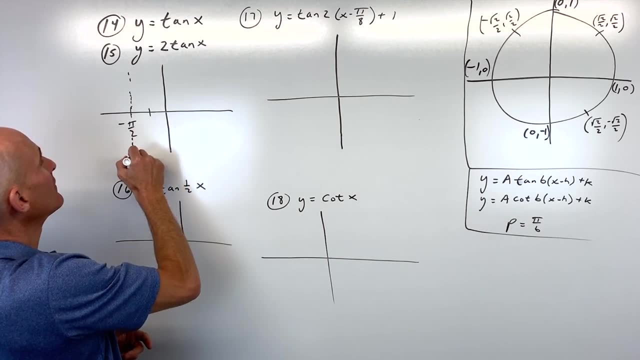 and tangent is y divided by x. Now negative 1 divided by 0, we can't divide by 0. That's undefined. So we're going to get a vertical asymptote right Here at negative pi over 2.. Now, at negative pi over 4, tangent's y over x- Anything divided. 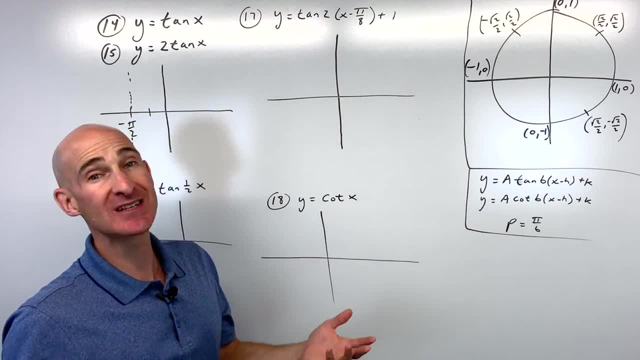 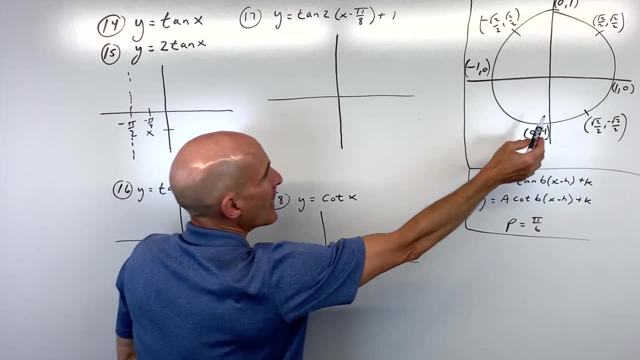 by itself is 1, but we have a negative divided by positive, which is negative 1.. So over here at negative, pi over 4, this is going to be right here at negative 1.. At 0, y divided by x: 0. 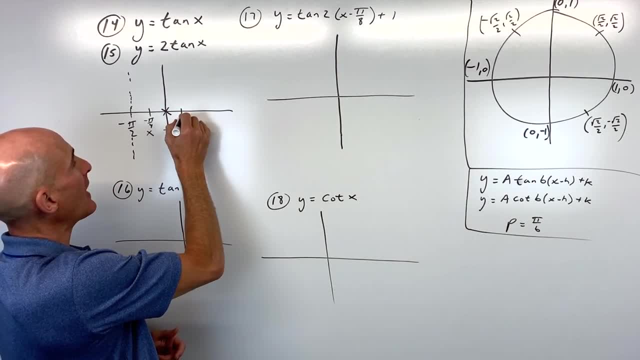 divided by 1 is going to be 0. So that's going to be another key point: At pi over 4, which is 45 degrees, tangent is y over x. Of course, anything divided by itself is going to be 1.. 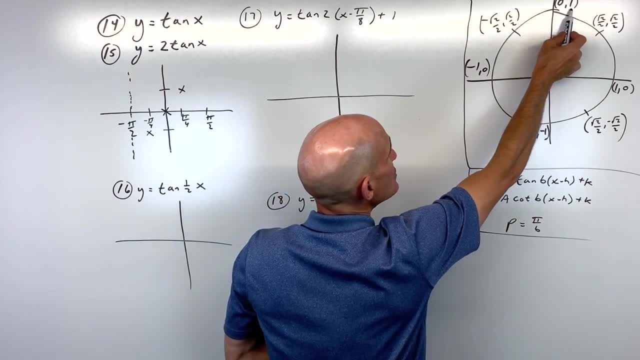 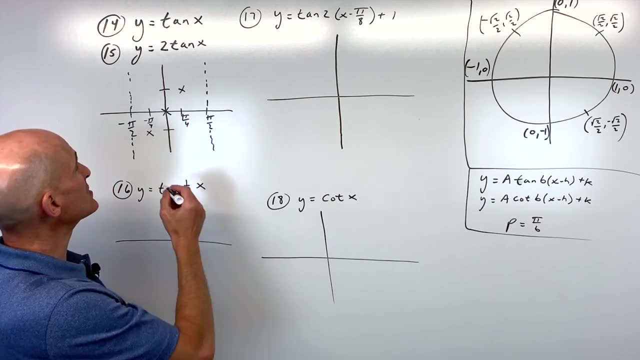 And then at pi over 2, tangent is y over x, 1 over 0. We can't divide by 0. That's undefined. We get another vertical asymptote. So that's one period. And what's interesting about tangent? 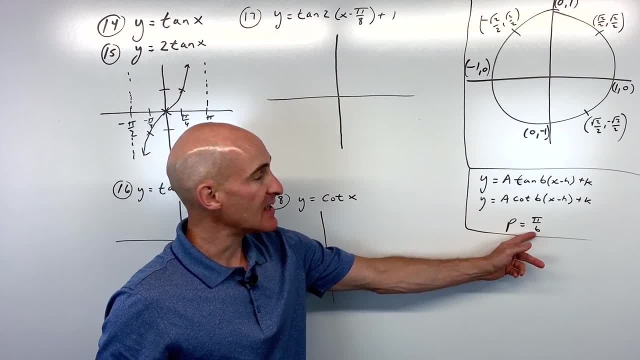 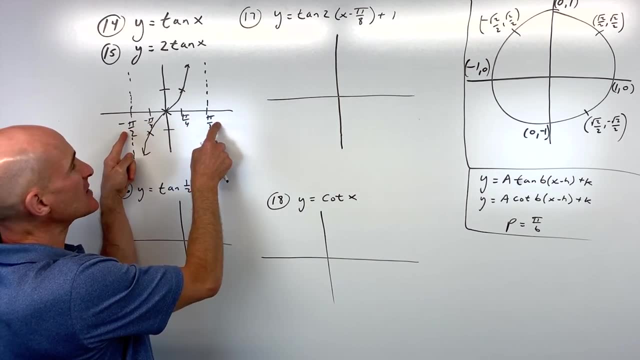 as opposed to sine and cosine is that the period is 1 pi divided by b, not 2 pi divided by b. So you can see that from negative pi over 2 to positive pi over 2, this is actually a period of pi. And then what happens is this graph is going to repeat like that, And then 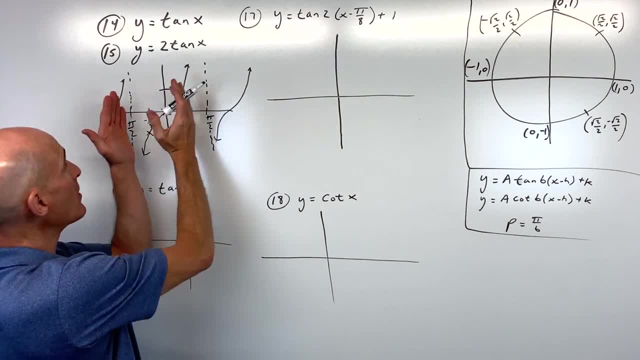 Same thing over on this side as well, and it's just going to keep repeating like that. But just one period, one cycle, from negative pi over 2 to positive pi over 2.. But for number 15, what do you think this 2 does to the graph? 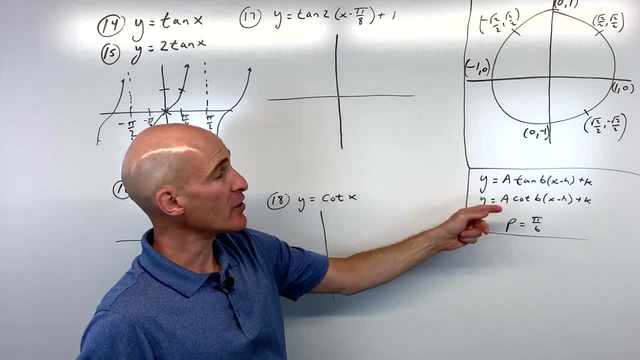 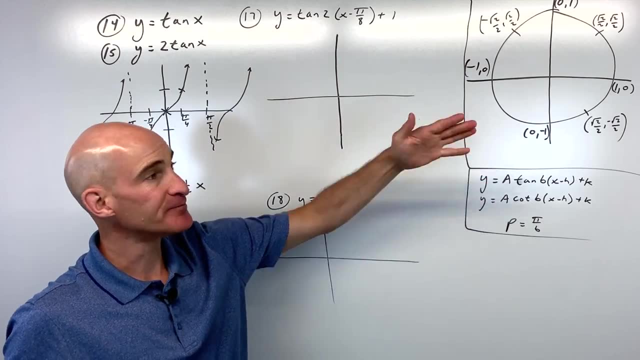 Well, you can see, the 2 is this coefficient in front here and it's going to be like a vertical stretch if it's greater than 1, or a vertical shrink if it's between 0 and 1.. Of course, if it's negative, that's going to reflect it over the x-axis. 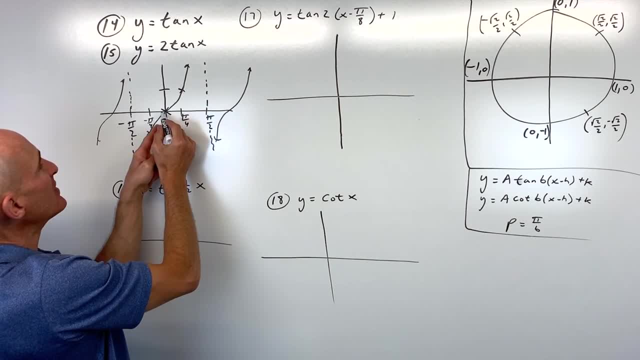 So if I was to graph a number 15 on this same graph, what would happen is: 2 times 0 is still 0.. Well, 1 times 2 is going to give us 2, and negative 1 times 2 is going to give us negative 2.. 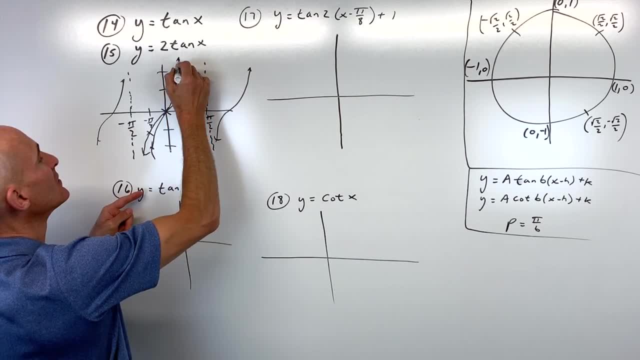 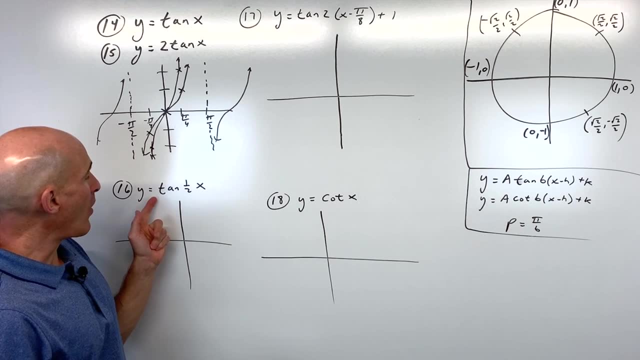 So what would happen here is the graph would actually be something like that: where it's being stretched, It's going up faster, 2 times faster. Okay for number 16,. we've got y equals tangent of 1 half x. 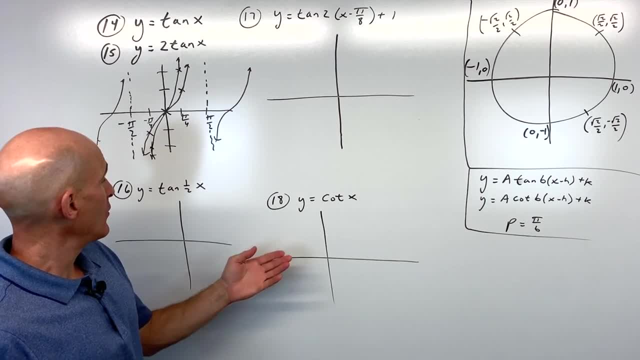 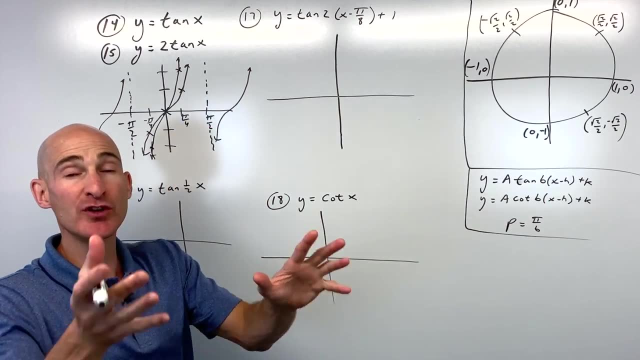 What do you think the 1 half does to the graph? Well, you can see that this number here is in front of our variable x, That's our b value, pi divided by 1 half. Remember, when you divide by a fraction, it's like: 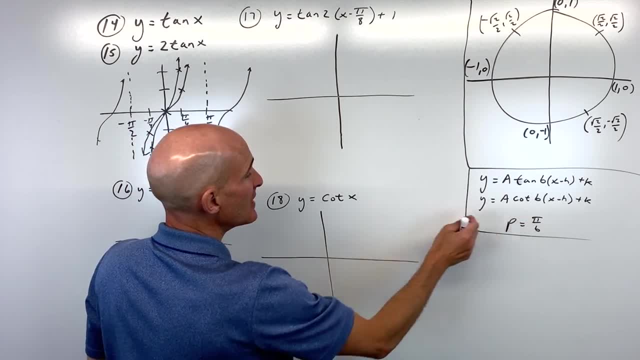 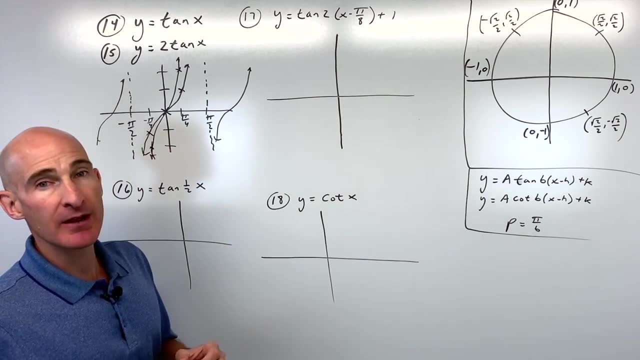 I'm multiplying by the reciprocal, so that means that this period is actually going to be not a half, but actually doubled. It's actually going to be 2 pi. Now, when you graph tangent, an important thing to realize is that see how half the graph is to the left of the y-axis and half the graph is to the right. 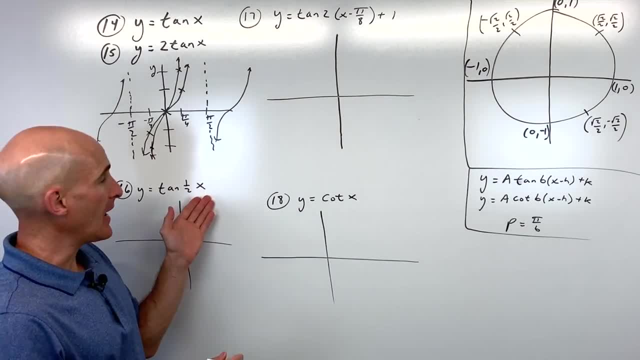 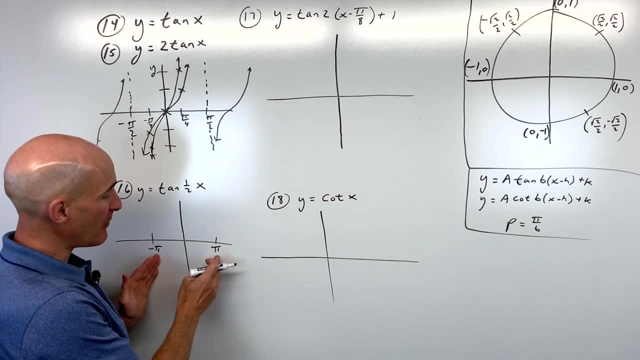 So when you figure out what the period is like- in this case we figured out the period is 2 pi- I'm going to cut that period in half, So half of 2 pi is going to be 1 pi and I'm going to put negative pi. So from negative pi to pi, that's actually a period of 2 pi. 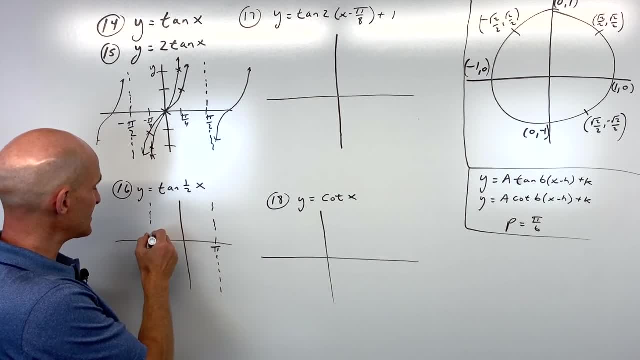 right. So I'm going to go ahead and sketch in our asymptotes, okay, just as dotted lines. And then what I like to do is I like to cut this in half again. So half of pi is going to be pi over 2.. Some people call these like the halfway points or the midway points, and negative pi over 2.. 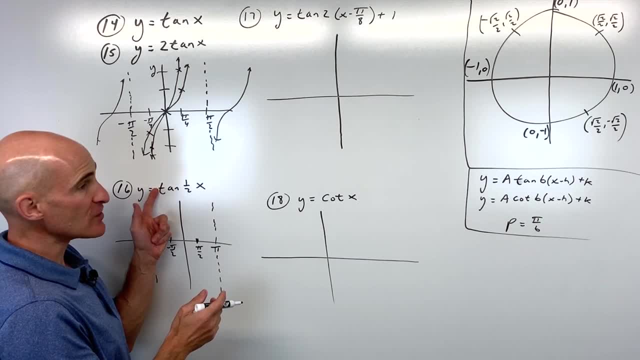 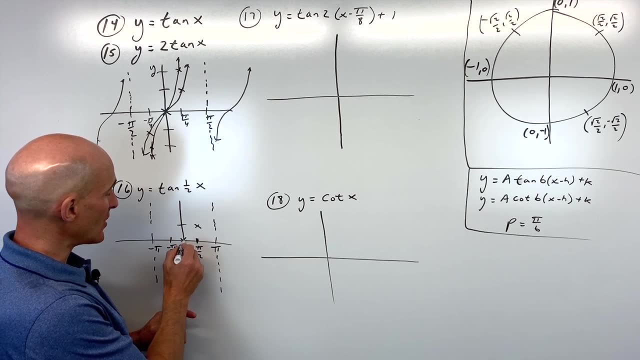 Okay. so now what we're going to do is: you can see that this coefficient in front of the tangent is just 1.. So we're just going to be going at these halfway points up to 1 and then down to negative 1, and it goes right here through the origin and we've got a good sketch of our graph. 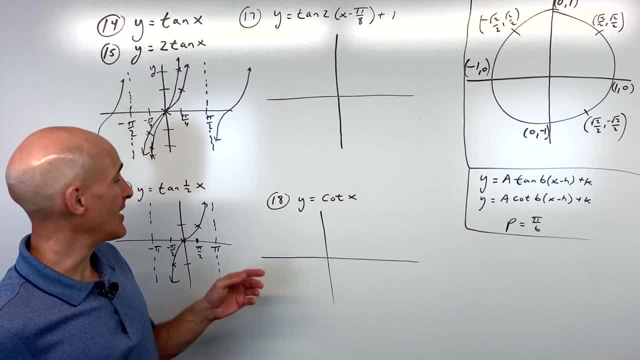 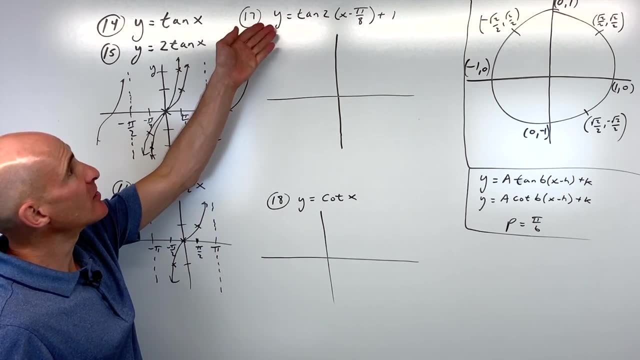 So remember the one that's, This group with the x actually has the opposite effect. It looks like we're dividing by 2.. We're actually multiplying the x values by 2, and that's stretching it horizontally. Let's look at another example, number 17.. This one has more going on here. The first thing I 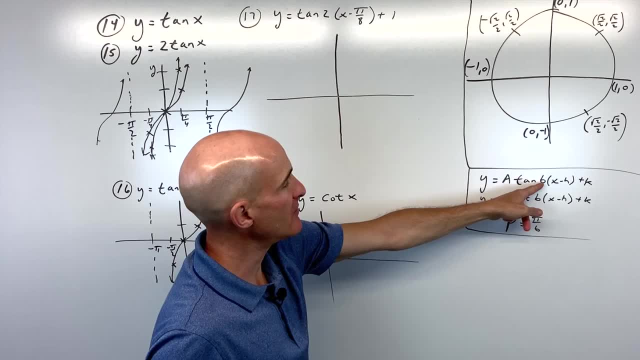 like to do is figure out what the period is. So I would look at that coefficient, that b value, and I'd say, well, let's see pi divided by 2, that's pi over 2.. But again, because half's on. 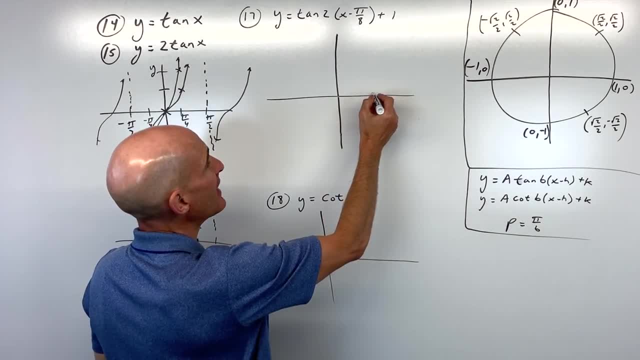 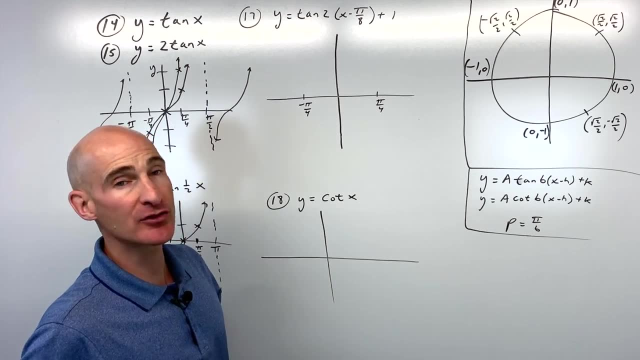 the left and half's on the right side of the y-axis. what we're going to do is we're going to cut it in half again, making this pi over 4.. And negative pi over 4, which gives us a period of pi over 2.. You can cut it in half again. 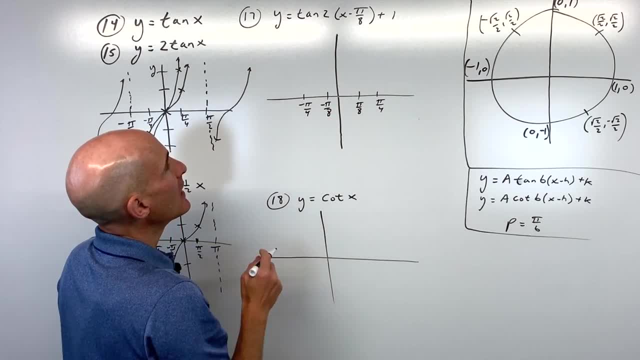 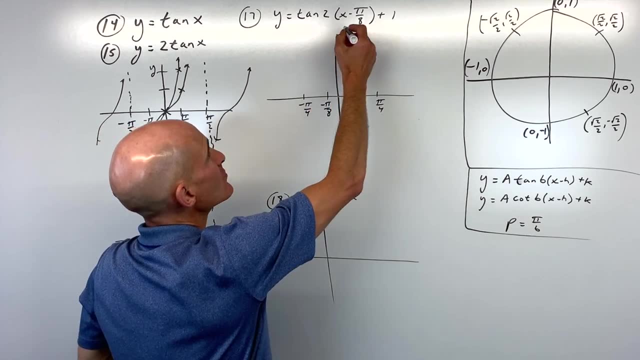 pi over 8, and negative pi over 8.. And then now let's look at the phase shift, okay, the left and right and the vertical shift up and down. So the number of this group with the x- remember this- has the opposite effect. The minus pi over 8 is actually going to shift it to the right pi. 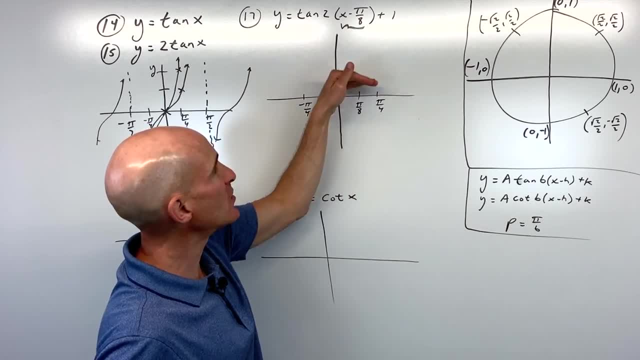 over 8,. okay, positive pi over 8.. And this one has the same effect. The plus 1 is going to shift it up 1.. But what I'm going to do in this one a little bit different than some of the other problems that. 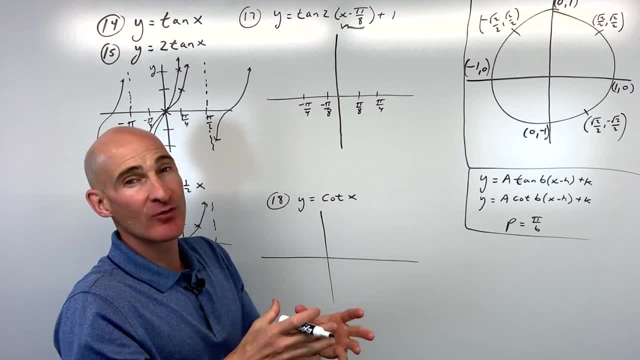 I've done in this video is I'm going to shift it to the right pi over 8. So I'm going to shift it up 1. And what I'm going to do in this video is: let's just graph what the original graph would look. 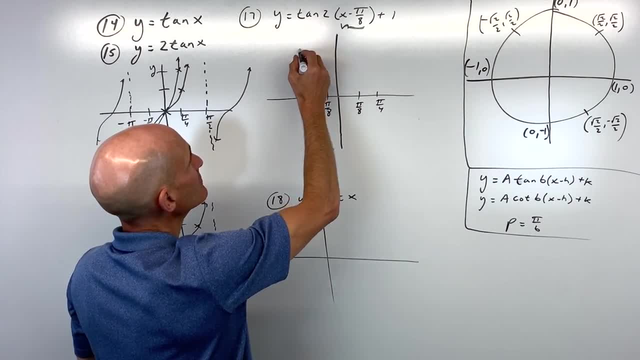 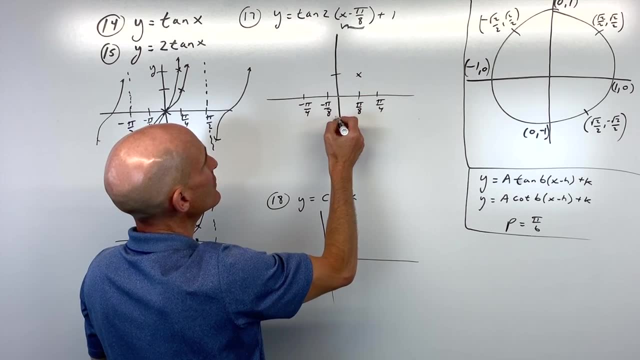 like without the shift. So we would have asymptotes right here. okay, like this and like this. But now what's going to happen is that it's going to go up here to 1,. it's going to go down here to. 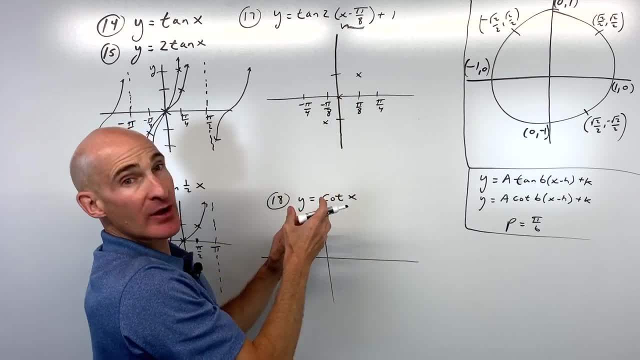 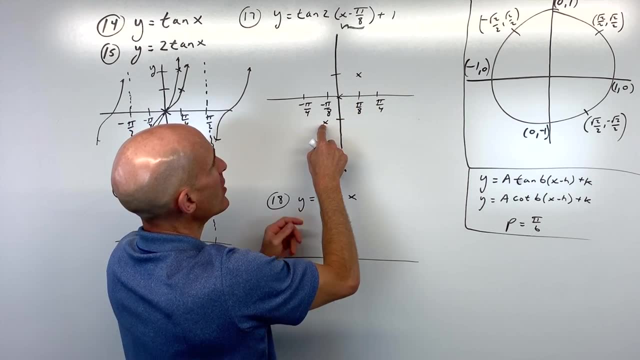 negative 1, and through the origin. But what the pi over 8 is going to do is going to shift it right, pi over 8.. So each of these points is going to move right, pi over 8, and then up 1.. So this point: 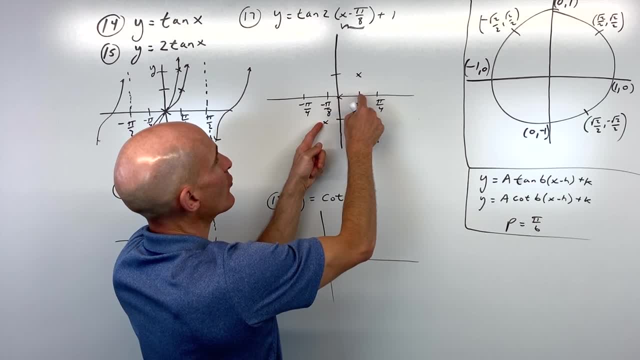 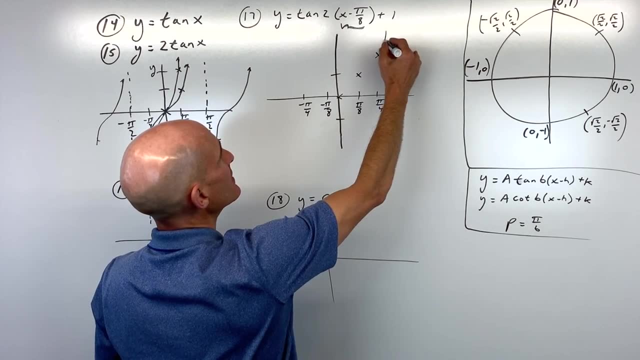 would go right here. and right here, This point is going to go right and up 1.. And this point is going to go right and up 1, like that. So now you can see, our graph is looking something like this: okay, And where our asymptote was here at negative pi over 4 is now: 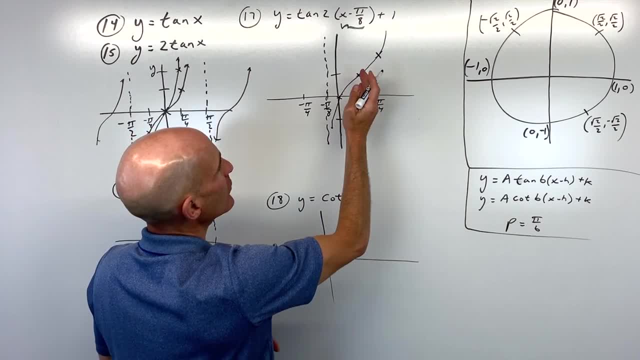 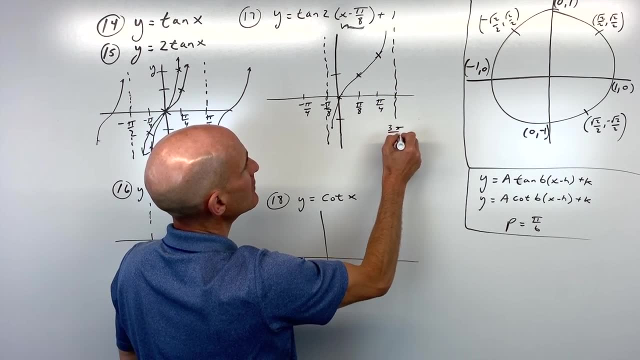 going to shift right pi over 8.. So it's going to be right here, And the one that was over here at pi over 4 is now going to be one step over here at 3 pi over 8.. And so now you've got your tangent. 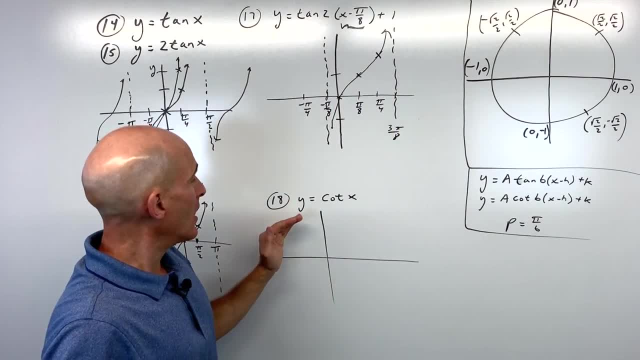 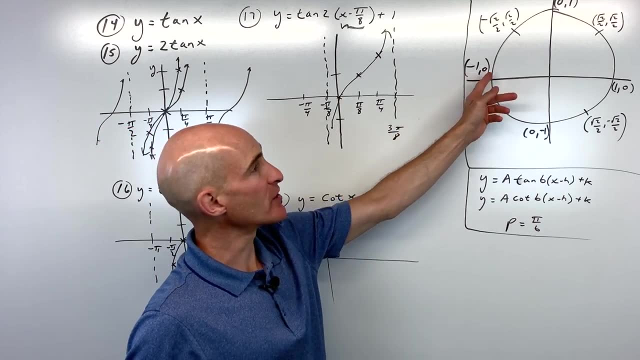 graph. So it shifted it right: pi over 8, up 1.. Okay, now let's take a look at cotangent. So when you think about cotangent, you're thinking on the unit circle. that's actually the x coordinate divided by the y coordinate And the unit circle values we're going to use for 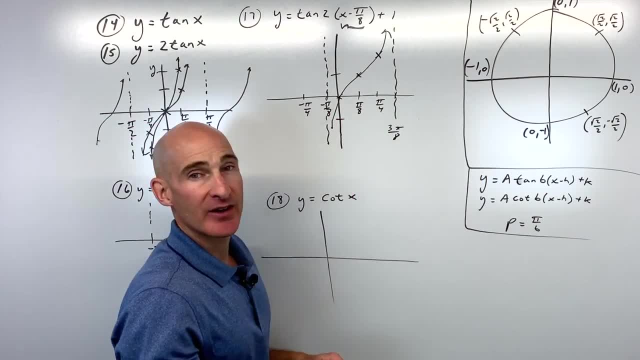 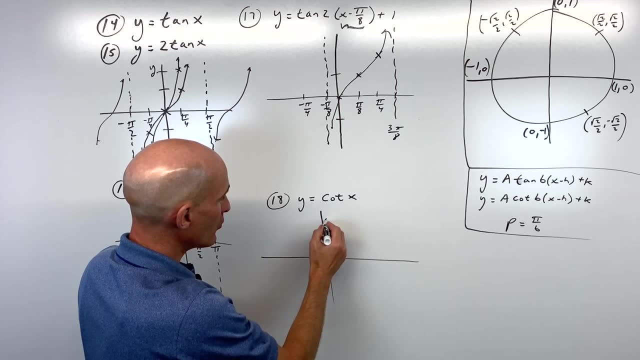 cotangent are from 0 to pi. okay, 0 to 180.. So cotangent of 0 is going to be 1 over 0, which is undefined. So right here, at 0, we're going to have an asymptote, okay, a vertical. 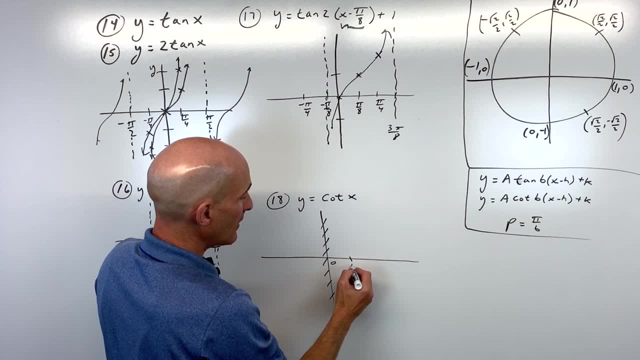 asymptote. At pi over 4, x divided by y is going to be 1, because anything divided by itself is 1.. And then over here we're going to have a vertical asymptote. So we're going to have a vertical. 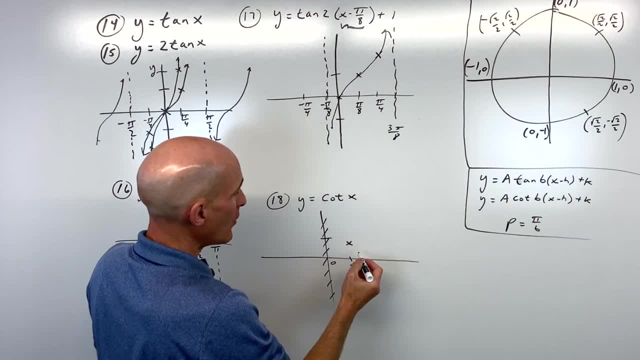 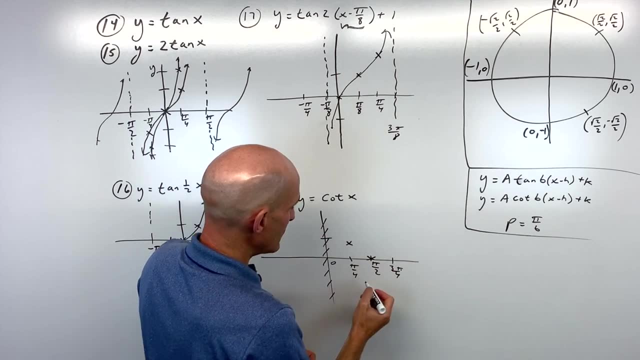 asymptote: Over here at pi over 2, x divided by y, 0 divided by 1 is going to be 0. Okay, and then over at 3. pi over 4, x divided by y is going to be negative 1.. And then over here at pi x divided by: 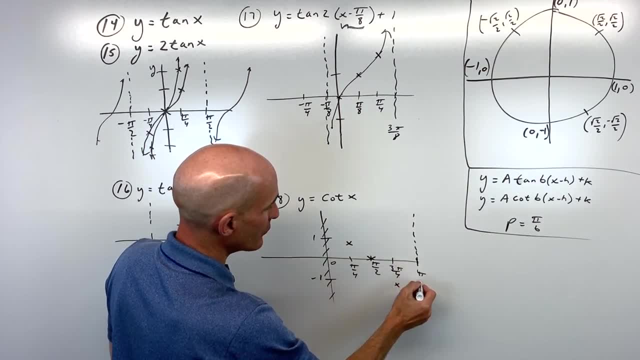 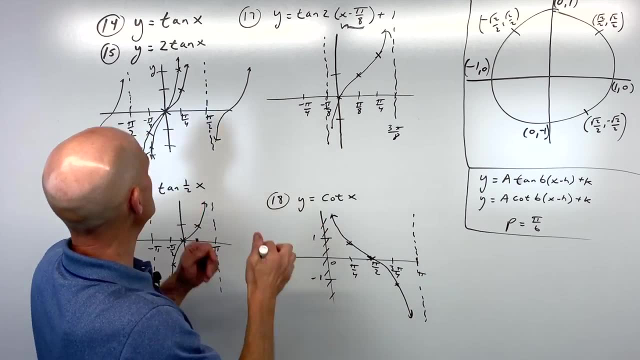 y negative 1 divided by 0 is undefined. So we get another vertical asymptote like that. So you can see the graph is going down to the right okay, whereas with tangent it was going up to the right. And the other interesting thing again. 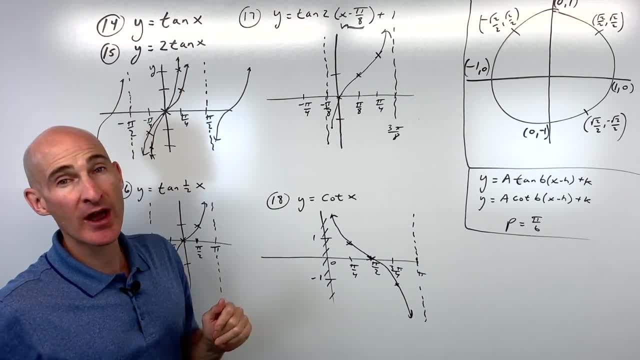 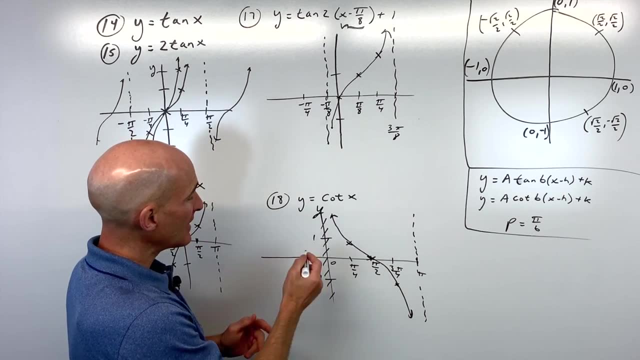 is that the tangent half of the graph is to the left of the y-axis, half is to the right, unless it's been shifted, Whereas with cotangent you can see that that whole graph is to the right of the y-axis. okay, But again the graph repeats, so there's going to be another branch over here. 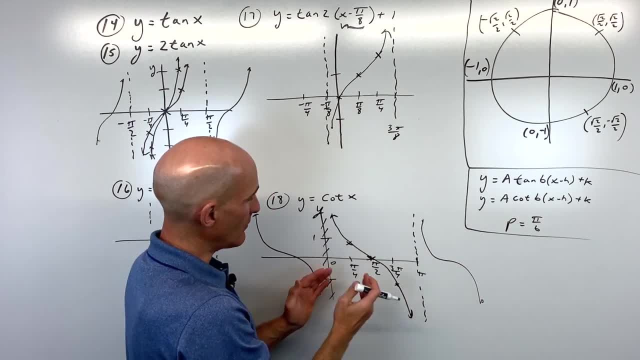 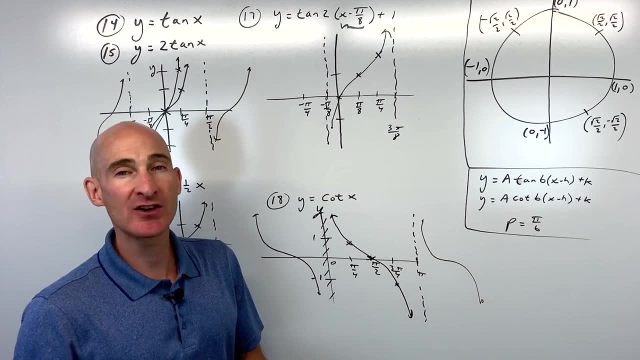 okay, another branch over here like that, and it's going to keep repeating, But for one period, one cycle, from 0 to pi, to the right of the y-axis, going down to the right is your basic graph. Let's look at a couple more challenging cotangent graphs. Okay, for number 19,. we have y equals 3. 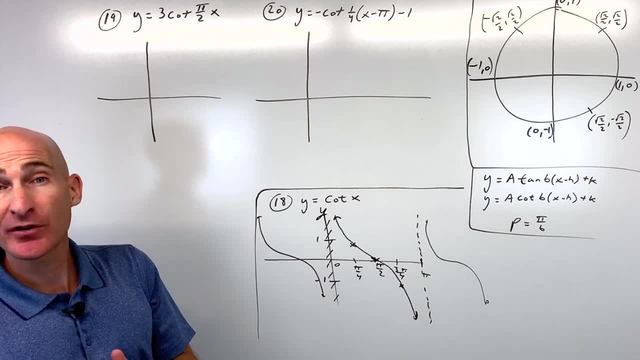 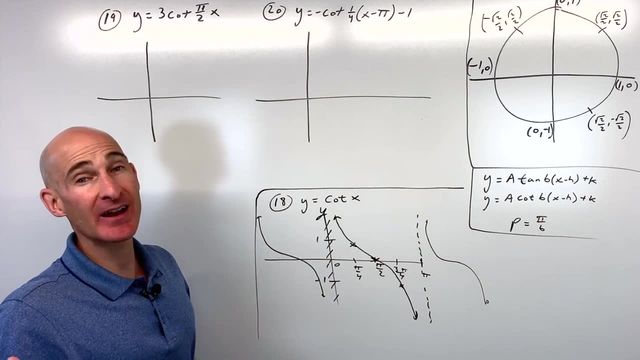 cotangent pi over 2, times x. So the first thing I like to do is to figure out what the period is using this formula. So for tangent and cotangent we're going to be using the period equals pi divided by b For sine. 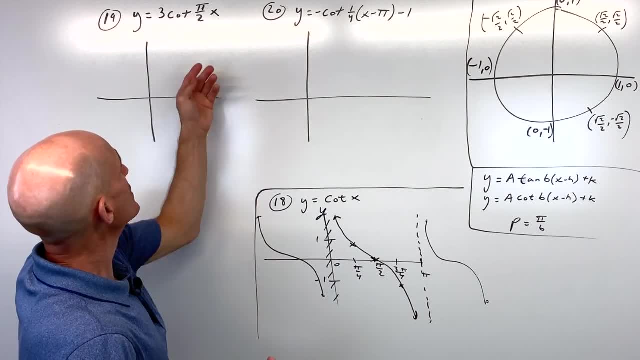 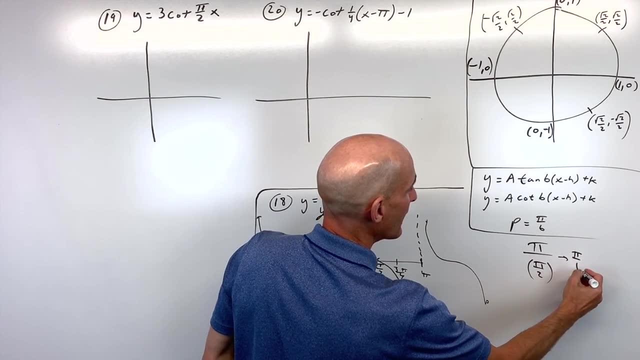 cosine, secant and cosecant, it's 2 pi divided by b. So if we do pi divided by pi over 2, that's really the same as pi times 2 over pi, because when you divide by a fraction, 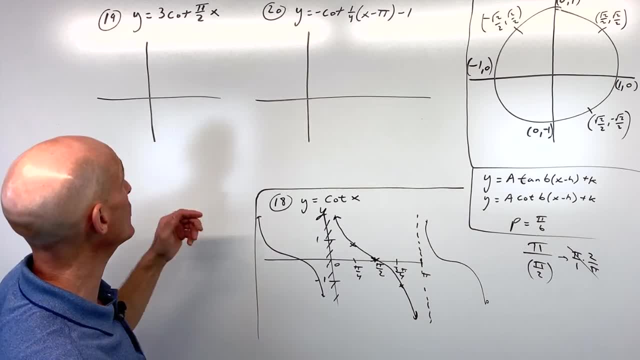 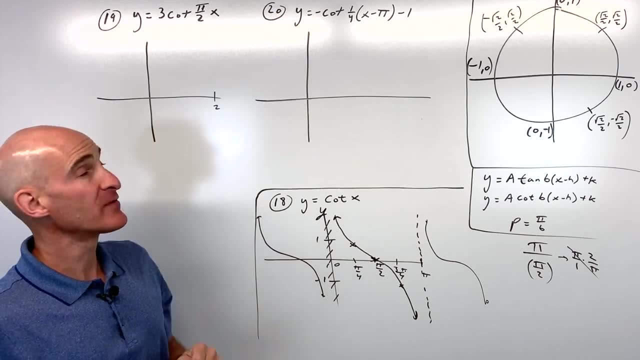 you're multiplying by the reciprocal Notice, the pi's cancel and we get a period of 2.. So there's no pi in the period here, just 2.. So what I'm going to do is I'm going to label this as 2, and if I divide this by 4, cutting it up into 4 pieces. 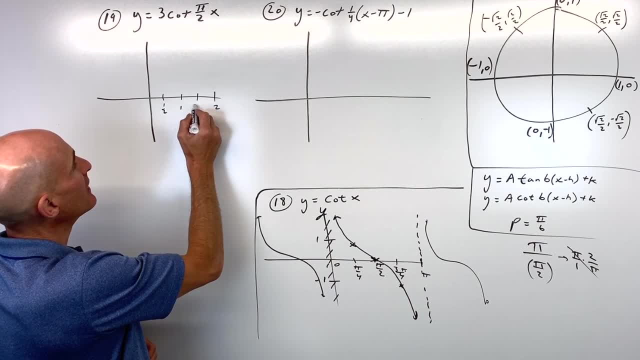 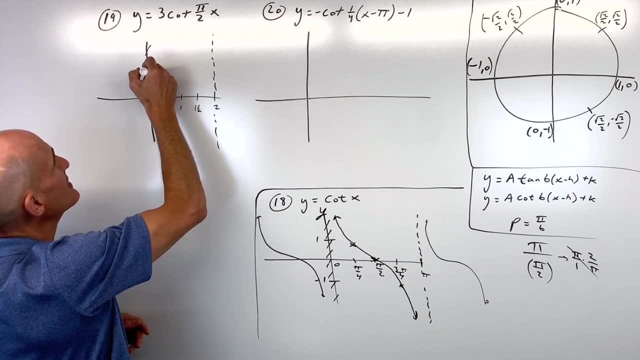 that's going to be 1 half 1, and 1 and a half. Okay, And so now you can see, our asymptotes are going to be right here at 2 and 0.. Okay, just like our parent function, right here. Okay, it hasn't been shifted at all. 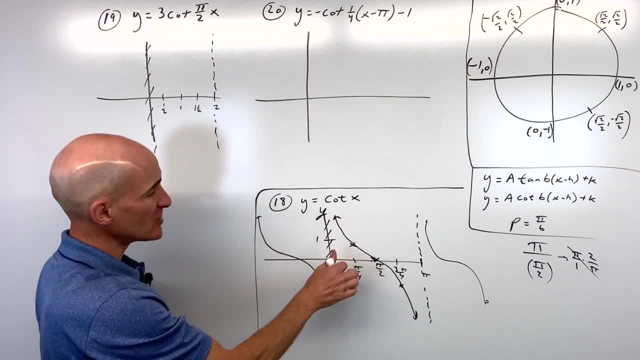 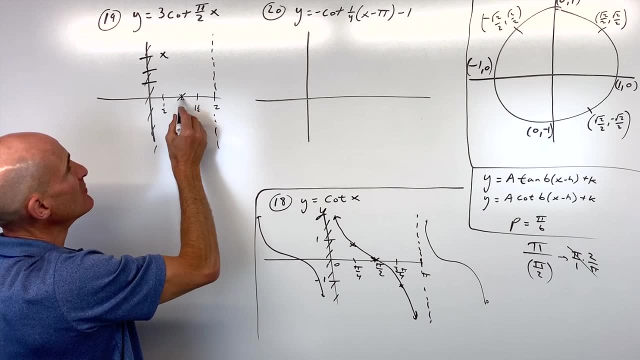 But what does the 3 do to the graph? Well, the 3 is going to be a vertical stretch, So this point here which is normally at 1, is now going to be at 3.. So, right there, Crosses at the midline here, And then this point here which is normally at negative 1,. 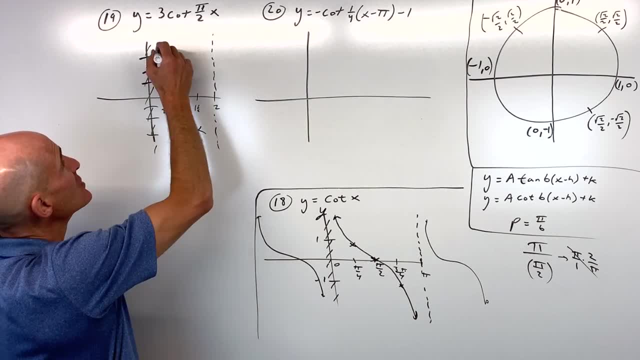 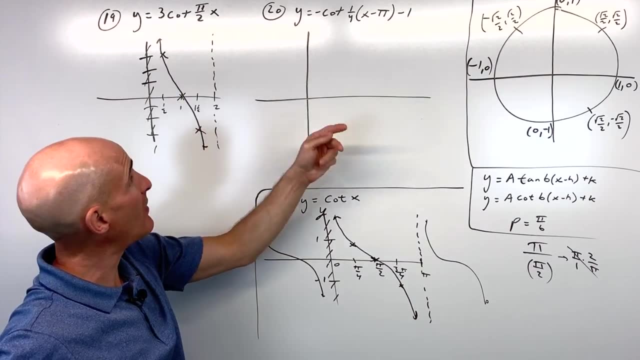 is going to be multiplied by 3. It's going to be at negative 3.. 1, 2, negative 3.. So you can see this was just a vertical stretch and then the period had changed using the pi over 2.. So let's look at number 20 now, A little bit more challenging still. 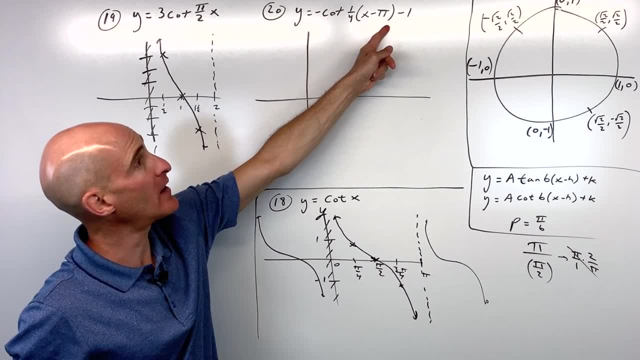 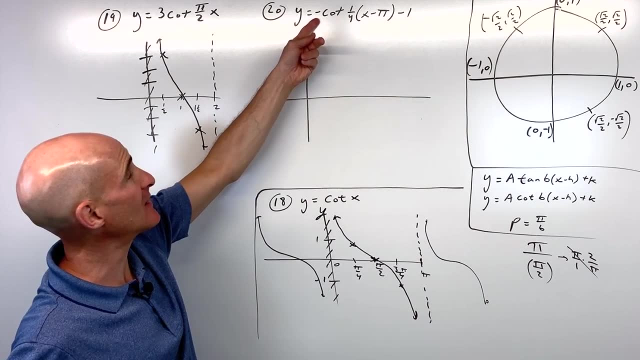 We've got: y equals negative cotangent 1. fourth, the quantity x minus pi minus 1.. Okay, so there's a lot involved in this one. The negative is going to reflect it over the x-axis. The y-value is the opposite sign, right? But let's figure out what our period is. I always do that first. 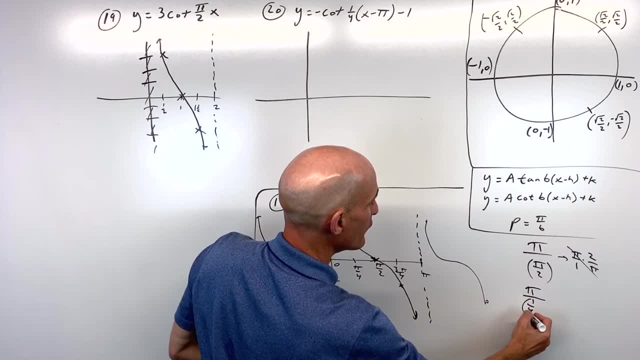 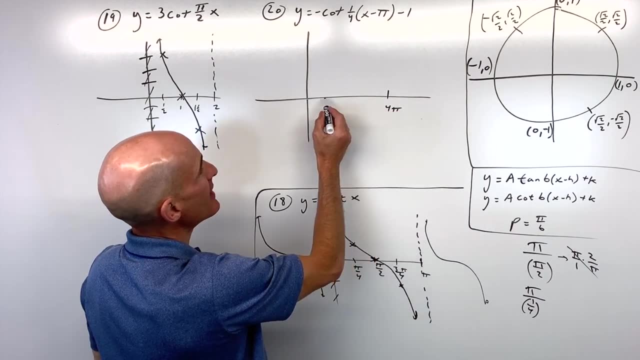 So I do pi divided by b. Now the b is 1 fourth. but when you divide by 1 fourth it's like multiplying by the reciprocal, So it's actually going to be 4 pi. So let's label this 4 pi. Let's divide it up into four pieces. 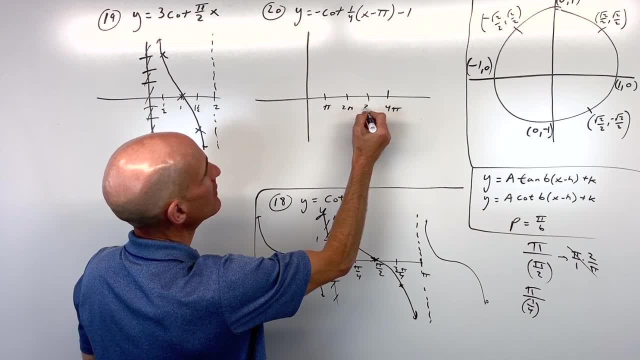 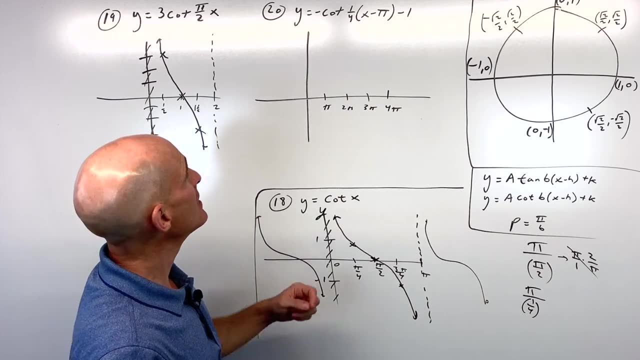 1 pi, 2 pi, 3 pi, 4 pi. And then now let's see: So normally cotangent is going down to the right, right, But the negative is going to reflect it, So now it's going to be going up to the right. So let's kind of just draw our basic graph here. 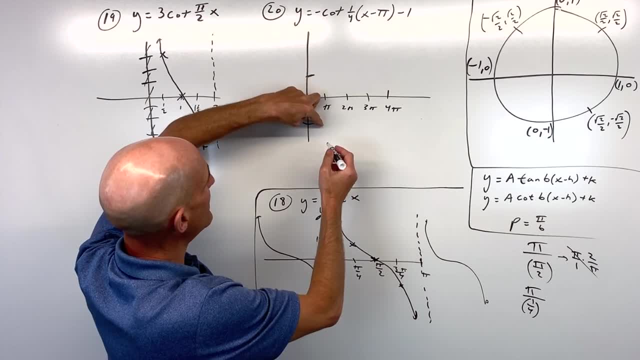 We're going to do it in two steps, So normally cotangent would be here. It's going to reflect, It's going to be down here at negative 1.. Crosses at the midline and then it goes up to positive 1,. 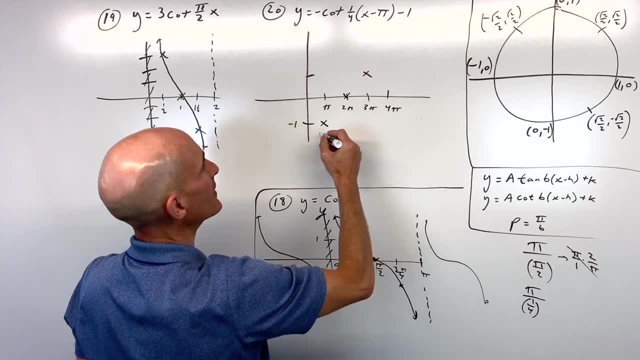 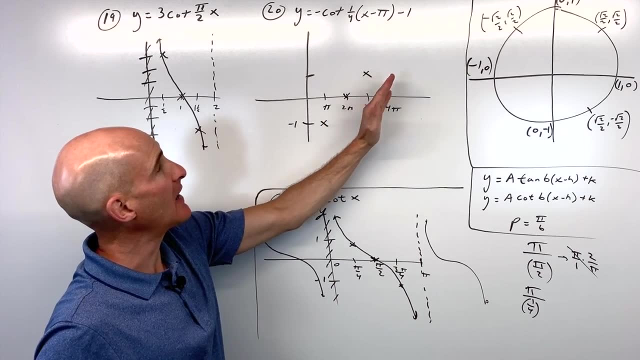 and then you have your other asymptote like that. So this would be your graph like that, right? But now what happens here? the minus pi and the minus 1? Well, this is actually going to have the opposite effect. It's actually going to go right: pi and the minus 1 is going to go down 1..